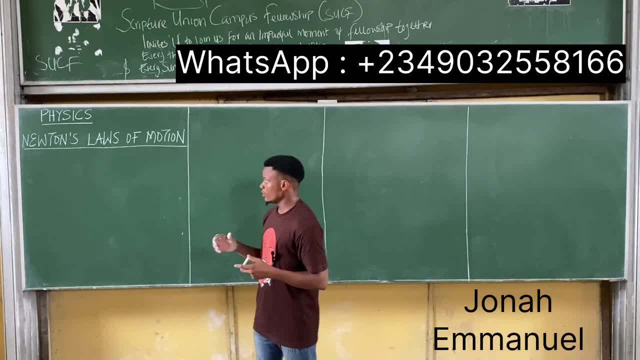 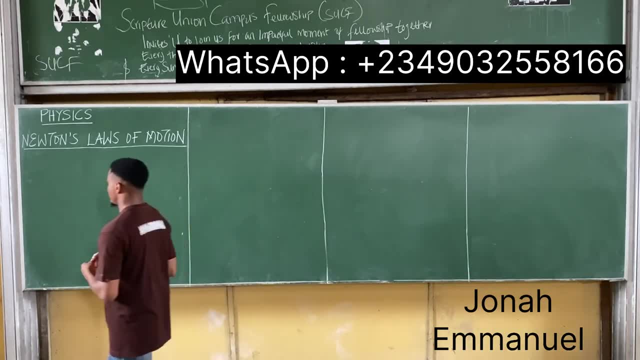 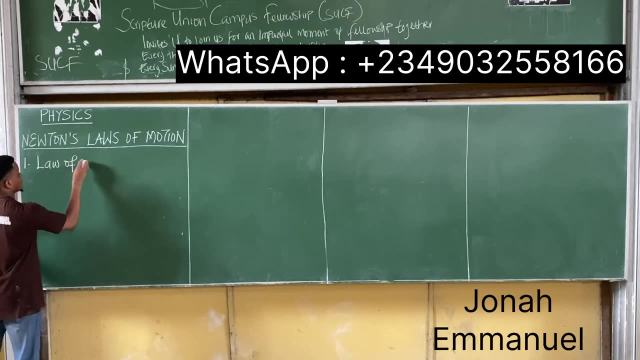 one or two of its application, All right. so one thing to notice is that Newton's Law of Motion was propounded by Isaac Newton and there are three. basically there are three laws under this. The first one is called the Law of Inertia, So Newton's first law. 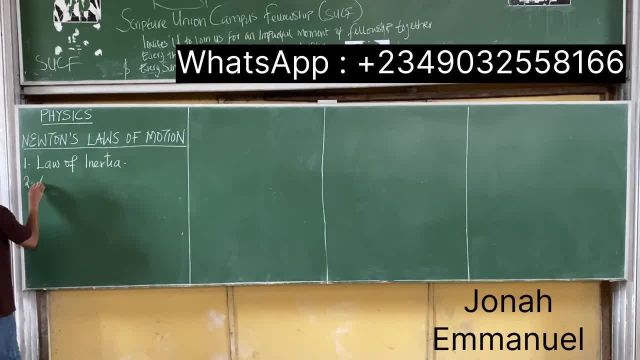 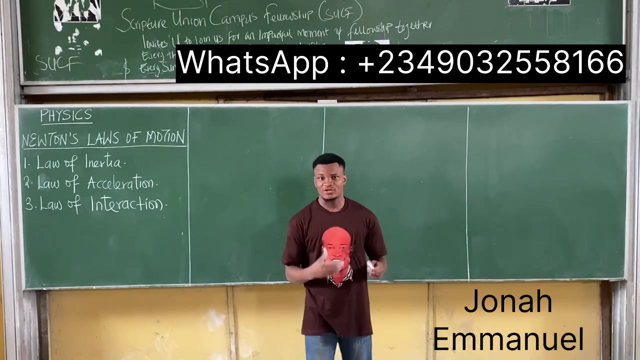 is called the Law of Inertia, Newton's second law is called the Law of Acceleration And Newton's third law is called the Law of Interaction. All right, so Newton's law can be stated as number one, the Law of Inertia, Number two, the Law of Acceleration. Number 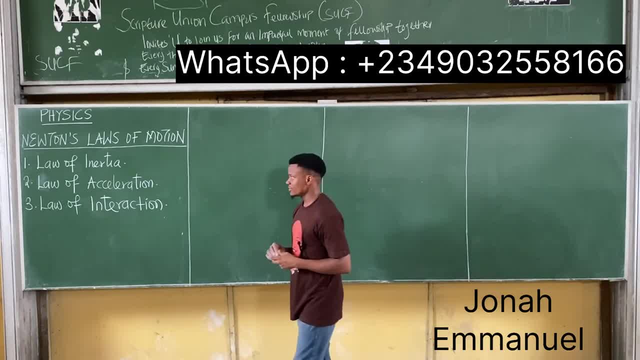 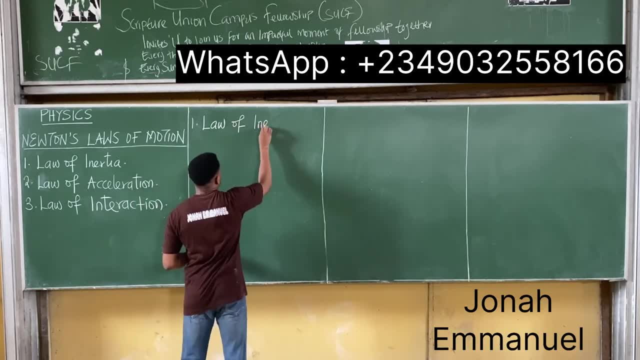 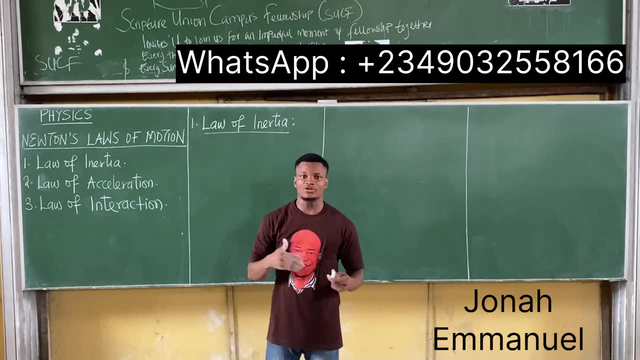 three, the Law of Interaction. So let's discuss this one after the other. Number one: let's look at Newton's first law of motion, called the Law of Inertia. So, by definition, Newton's Law of Inertia states that a body will continue in its state. 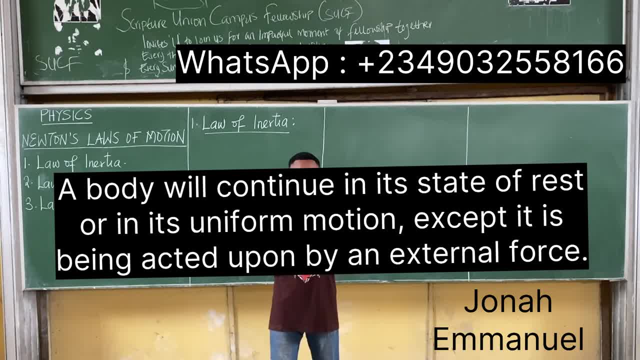 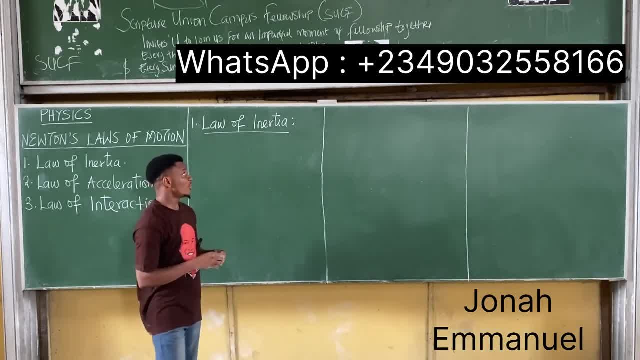 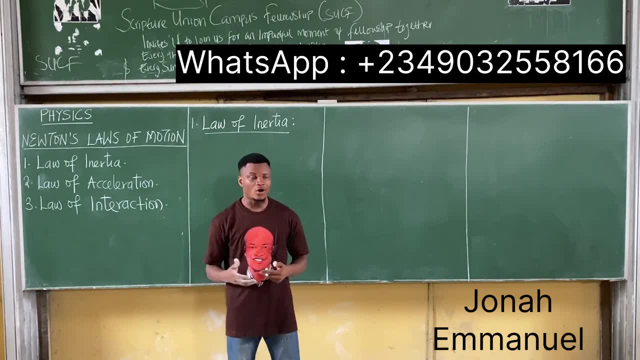 of rest or its uniform motion, except it is being acted upon by an external force. All right, that's a definition for Newton's Law of Inertia. all right, that a body will remain in its state of rest or its uniform motion- uniform motion, except it is being acted upon by an external force. all right now. 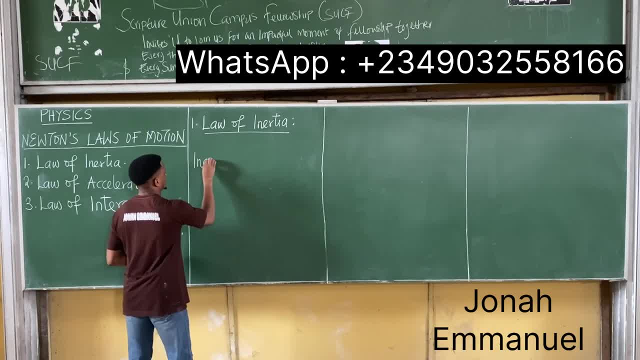 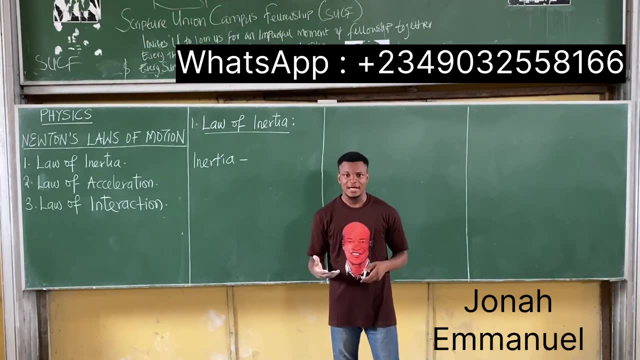 I will say love inertia. when we use the word inertia, always use the word inertia. what does the word inertia mean? inertia, by definition, right. inertia by definition is simply the tendency of a body at rest to remain at rest and the tendency of a body, of a moving body, to remain in motion. that's the concept of. 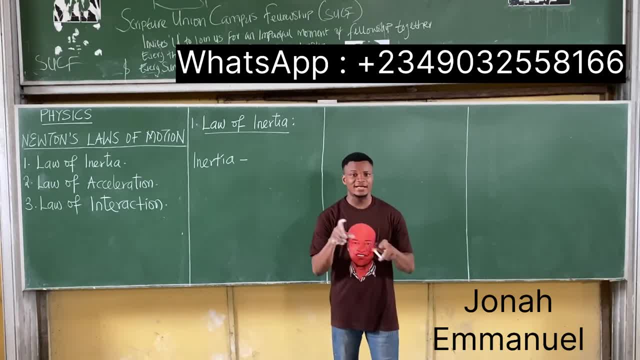 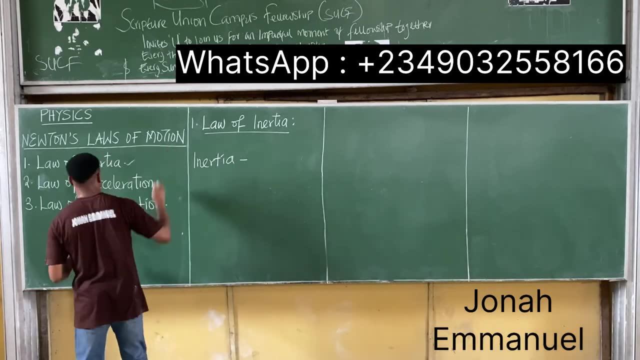 inertia. so, by definition, inertia is simply the tendency of a body at rest to remain at rest and the tendency of a body in motion to remain in motion. right, that's the idea of inertia. so that's the first law of inertia. that's how we state this. let's look at the second law, called the law Number 2. 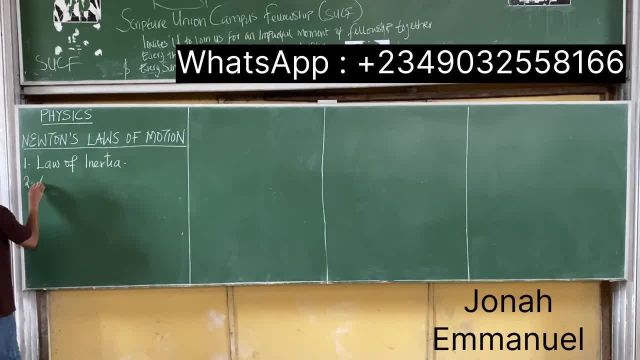 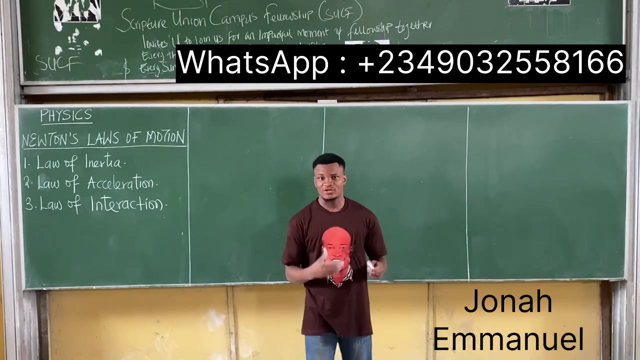 is called the Law of Inertia, Newton's second law is called the Law of Acceleration And Newton's third law is called the Law of Interaction. All right, so Newton's law can be stated as number one, the Law of Inertia, Number two, the Law of Acceleration. Number 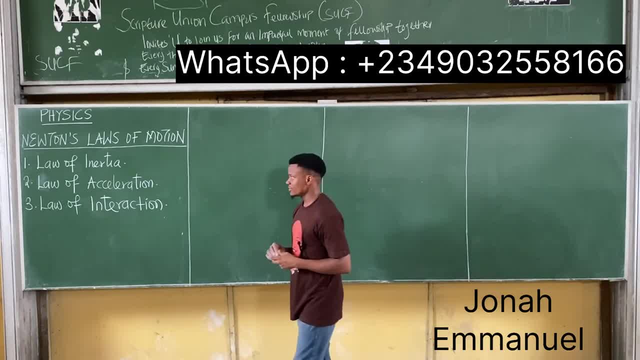 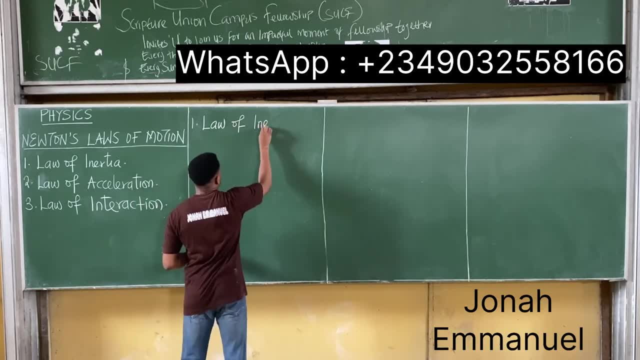 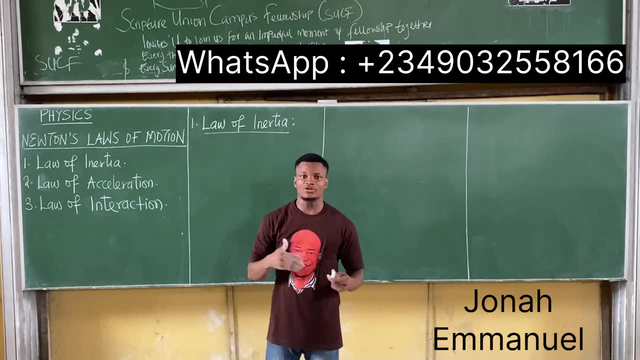 three, the Law of Interaction. So let's discuss this one after the other. Number one: let's look at Newton's first law of motion, called the Law of Inertia. So, by definition, Newton's law of inertia states that a body will continue in its state. 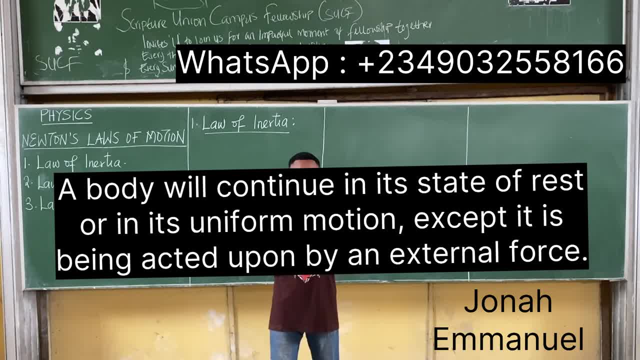 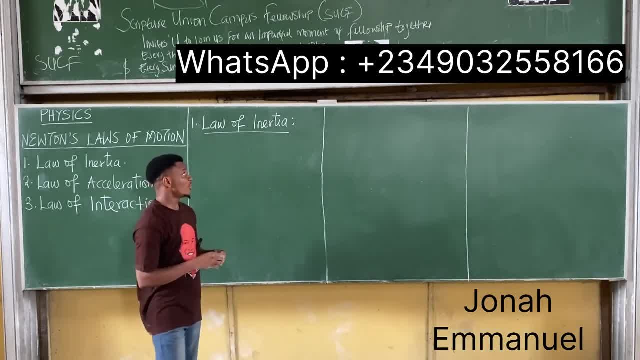 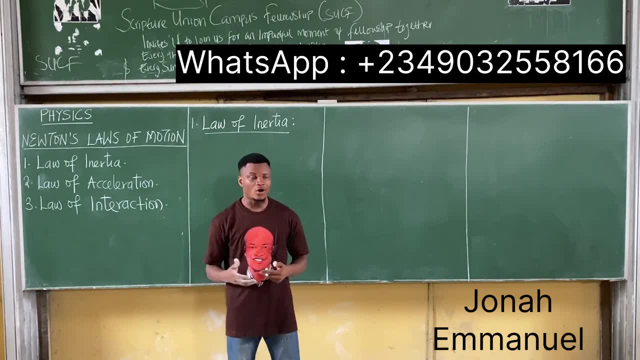 of rest or its uniform motion, except it is being acted upon by an external force. That's a definition for Newton's Law of Inertia, That a body will remain in his state of rest, uniform motion, except it is being acted upon by an external force. all right now. 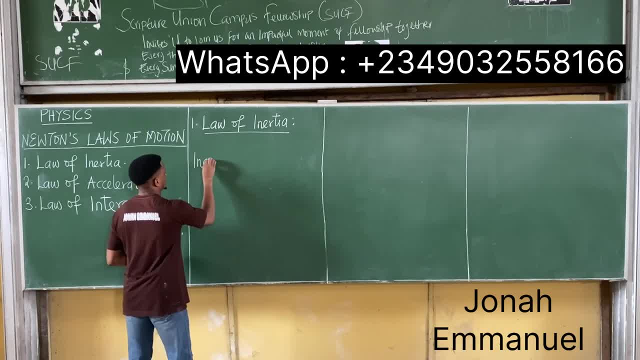 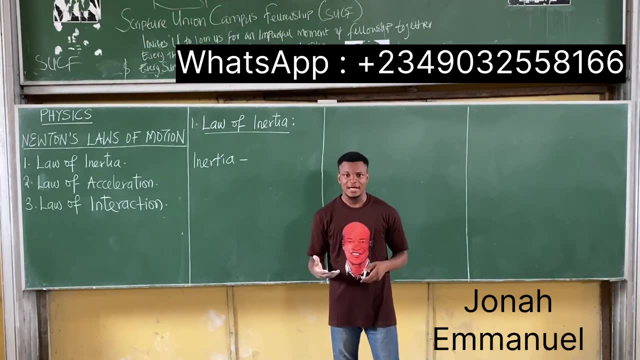 I will say love inertia. when we use the word inertia, always use the word inertia. what does the word inertia mean? inertia by definition, right. inertia by definition is simply the tendency of a body at rest to remain at rest and the tendency of a body or of a moving body to remain in motion. that's the concept of. 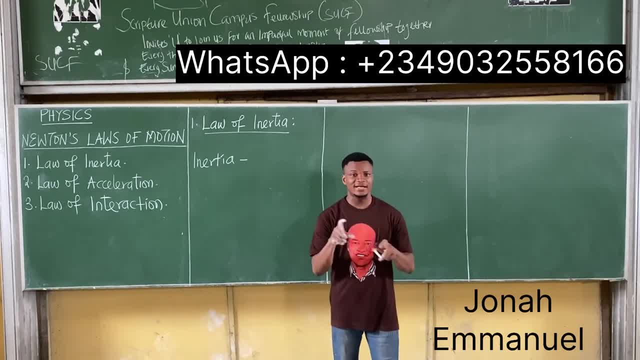 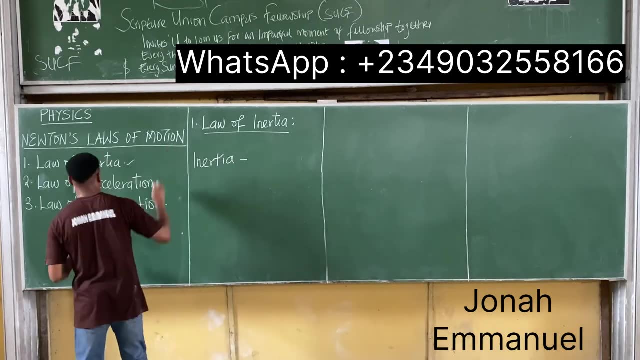 inertia. so, by definition, inertia is simply the tendency of a body at rest to remain at rest and the tendency of a body in motion to remain in motion. right, that's the idea of inertia. so that's the first law of inertia. that's how we state this. let's look at the second law, called the law number two. 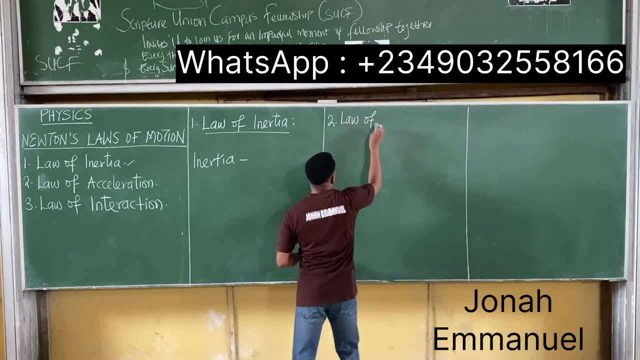 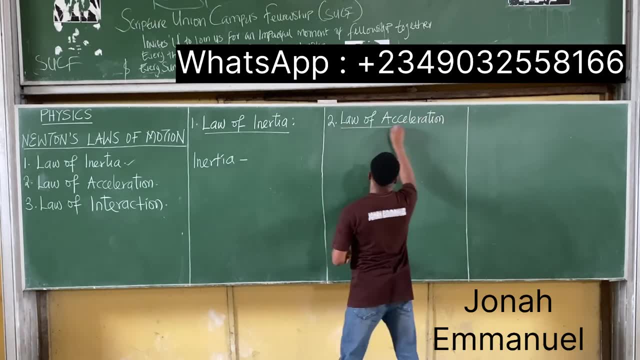 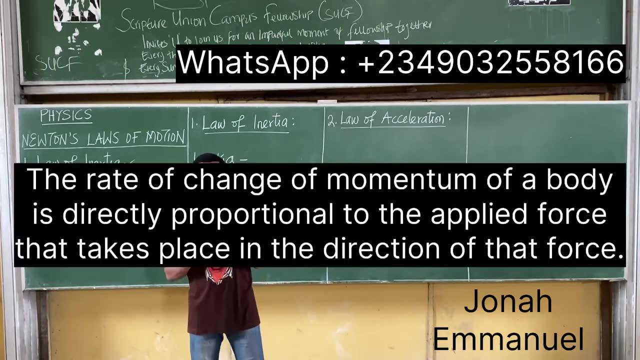 number two called the law of acceleration. all right, Newton's law of acceleration states that the rate of change of momentum of a body is directly proportional to the applied force that takes place in the direction of that force. that's how we state Newton's law of acceleration. 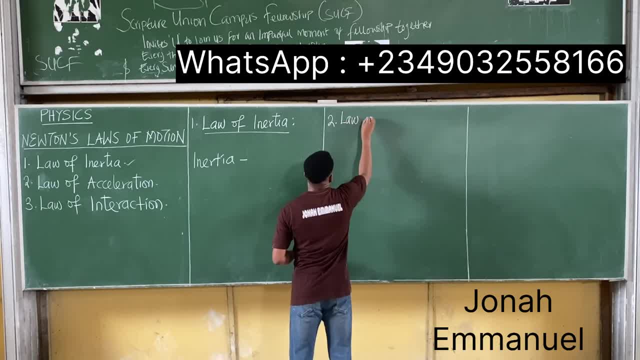 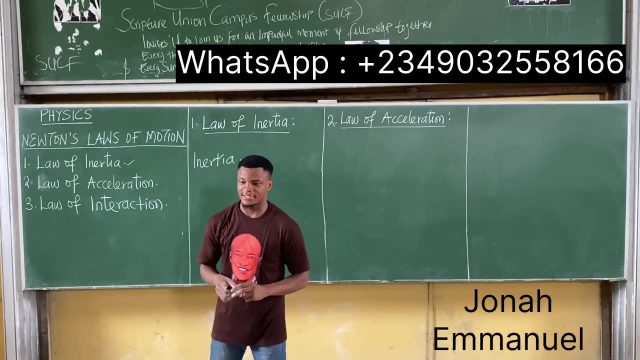 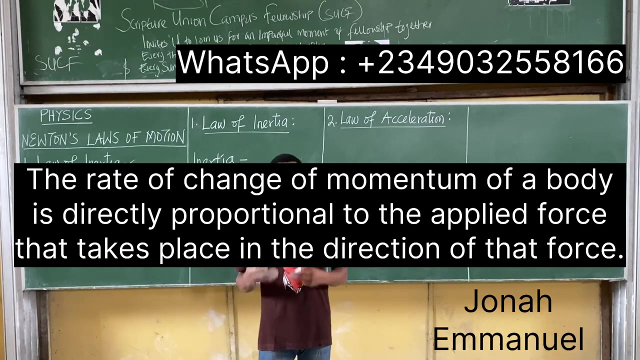 Number 2. It's called the Law of Acceleration. Acceleration, All right. Newton's Law of Acceleration states that the rate of change of momentum of a body is directly proportional to the applied force that takes place in the direction of that force. 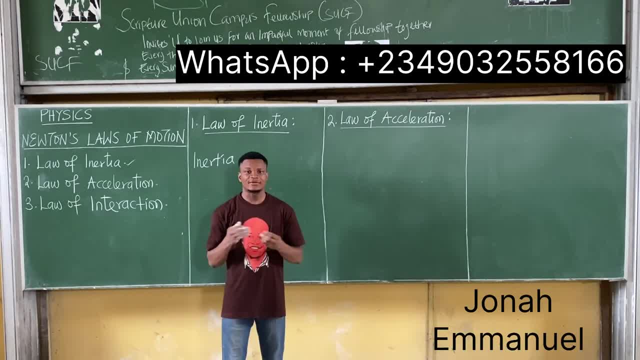 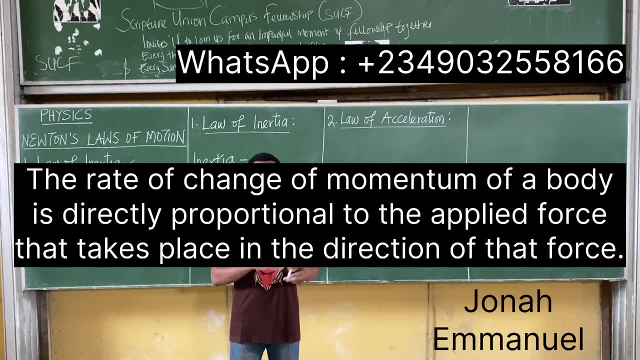 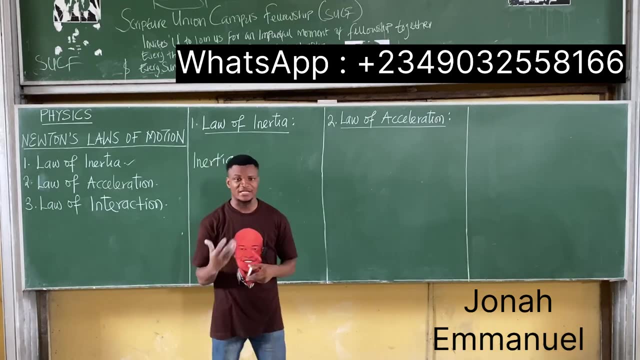 That's how he states. Newton's Law of Acceleration, That's, the rate of change of momentum of a body, is directly proportional to the applied force that takes place in the direction of that force. Okay, so Newton's Law of Acceleration actually has a mathematical expression. 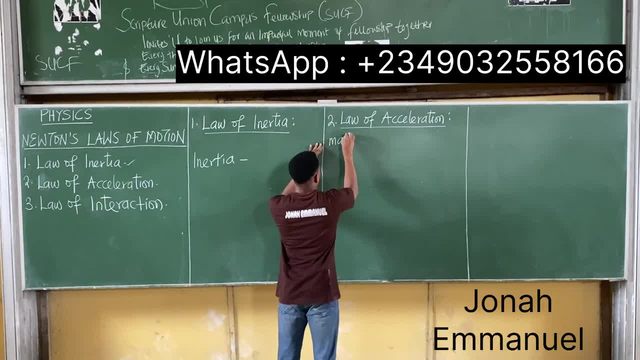 In mathematics form we have that. mathematically, we're saying that force we would have that force is. mathematically. we're saying that force is. mathematically. we're saying that force is directly proportional to rate of change of momentum. 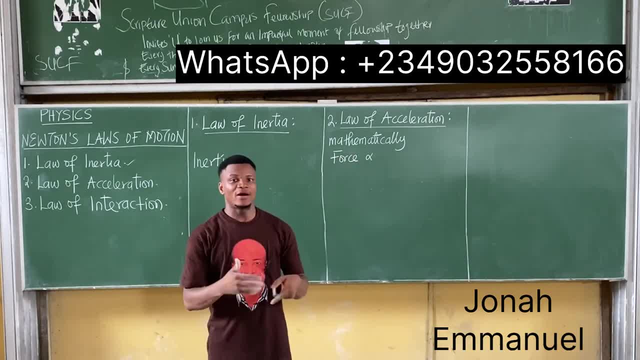 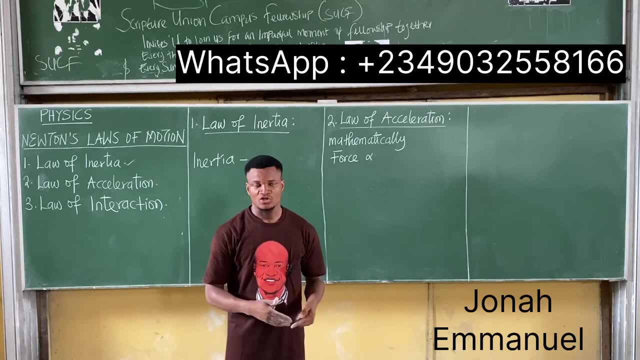 Now, when we say rate, the word rate is a time bound word. So when we say the rate of something, it means that thing is changing with respect to time. It becomes that thing over time. So if you now say the rate of change of momentum, it means momentum changing with respect to time. 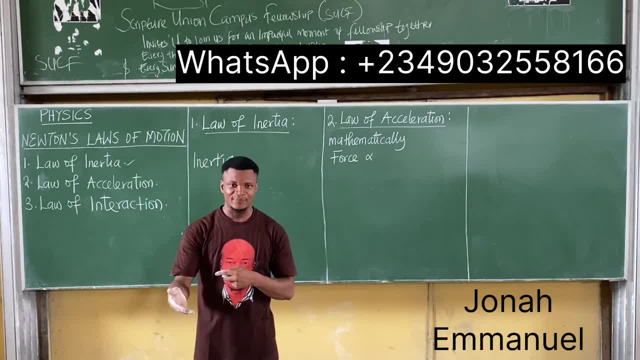 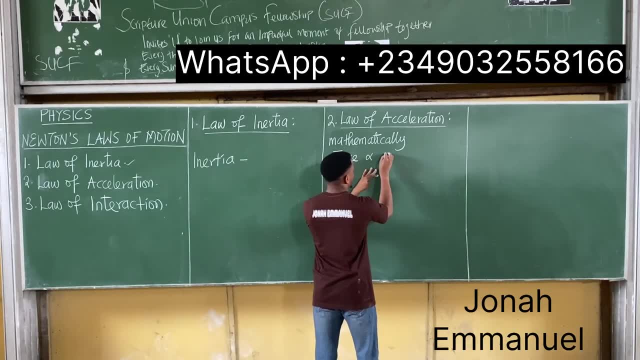 So the word rate always talks about how fast or how slow something is changing And hence the word rate is changing with respect to time becomes time. so we say rate of change of momentum. that becomes change in momentum all over time. this becomes rate of change of momentum, all right rates. 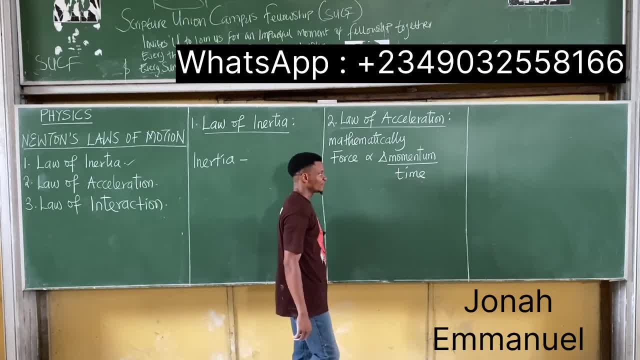 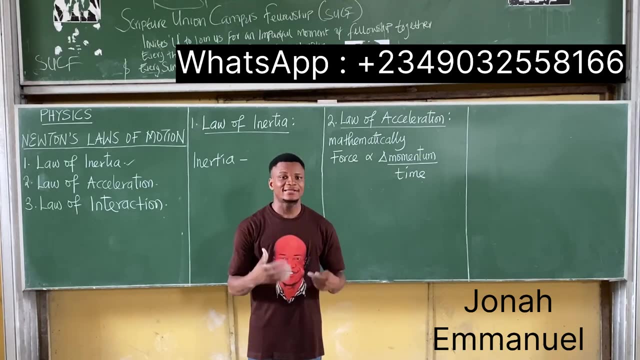 showing time, then change in momentum. so I have this now. the question would be this: if you look at the law of acceleration critically, we said that the rate of change of momentum is directly proportional to the applied force that takes place- or takes, yeah, that takes place- in the direction of that force. so 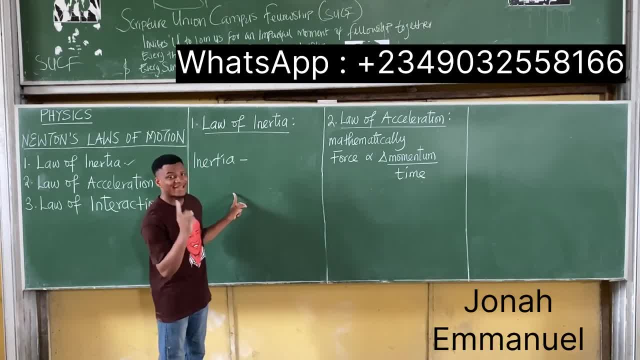 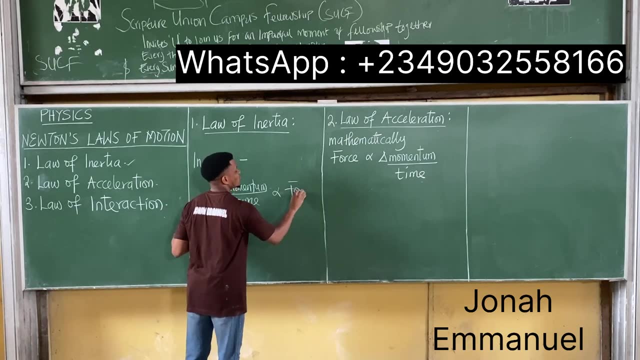 from that definition we have that the rate of change of momentum first being directly proportional to the force. so if I should consider that I should be having change in momentum, or perhaps rate of change of momentum being directly proportional to force, this is what I should have. I should have that. 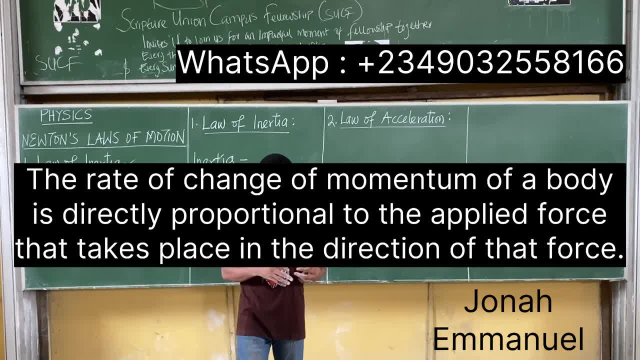 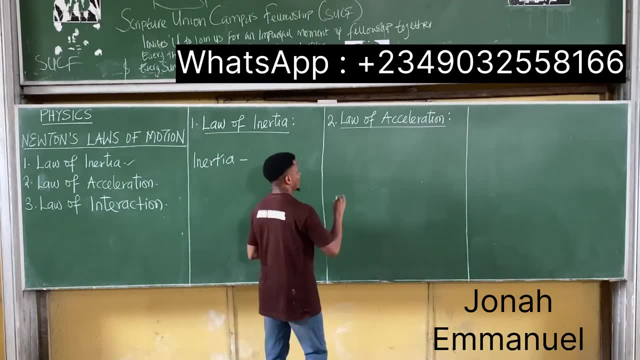 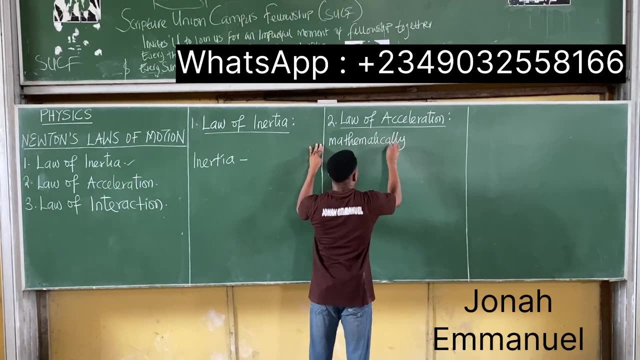 that's, the rate of change of momentum of a body is directly proportional to the applied force that takes place in the direction of that force. okay, soesters, love. acceleration actually has a mathematical expression in mathematics form. we have that in Mar C, Martin Preesار. we're saying that past would have does. 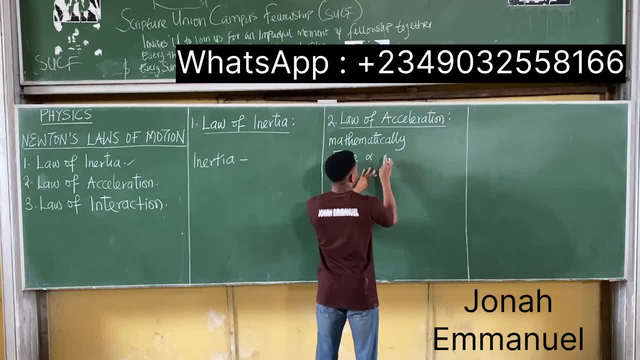 force it's slow because man goes forward or doesn't go ahead. basically, when a force change occurs, we get a momentum expression and that rates changes, that the somehow新s law of acceleration actually has a mathematical expression. in mathematics form we have that is directly proportional to rate of change of momentum. now when we say rate the 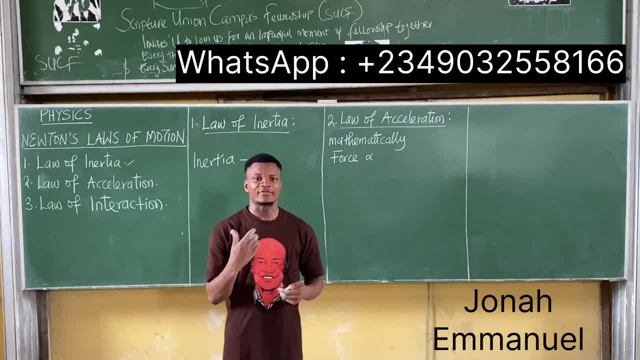 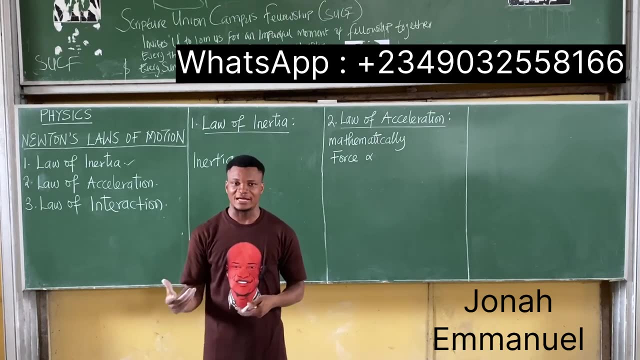 word rate is a time-bound word. so when we say the rate of something it means that thing is changing with respect to time. it becomes that thing over time. so if you now say the rate of change of momentum, it means momentum changing with respect to time. so the word there rate always talks about how fast or how slow. 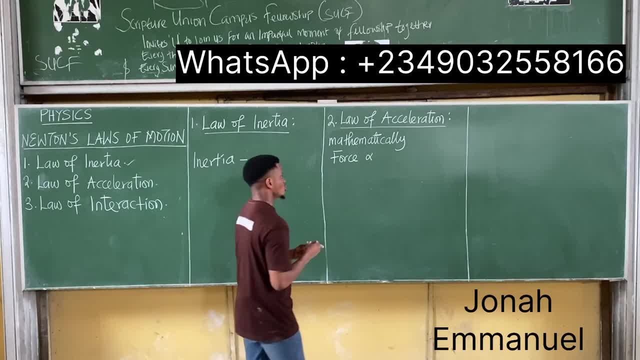 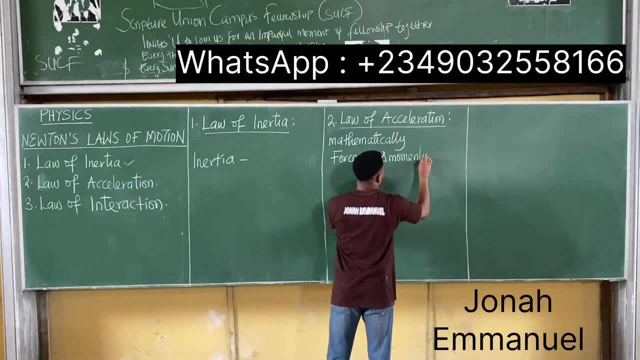 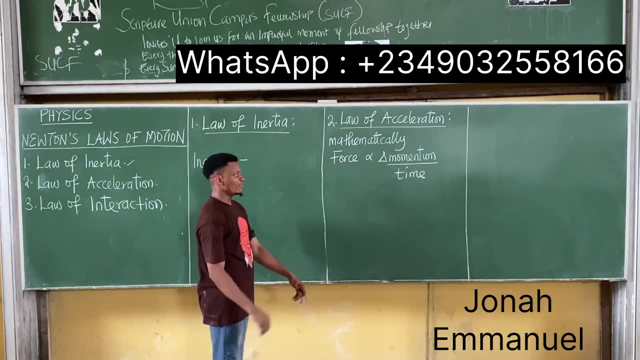 something is changing and hence becomes time. so if we say rate of change of momentum, that becomes change in momentum all over time. this becomes rate of change of momentum. all right rates showing time, then change in momentum. so I have this now. the question would be this: if you look at the law of acceleration, critically. we say that rate of change of momentum is the rate of change of. we say that the rate of change of momentum is directly proportional to the applied force that takes place or takes- yeah, that takes place- in the direction of that force. so from that definition we have that: the rate of change of momentum. 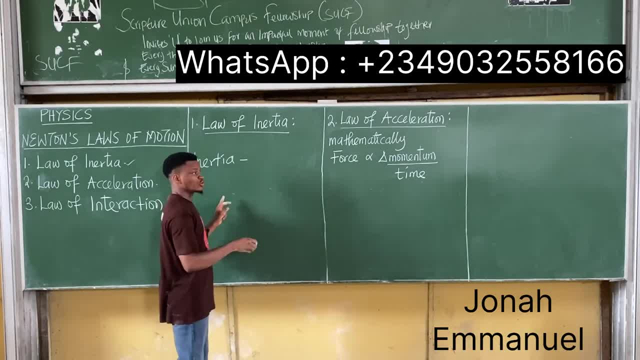 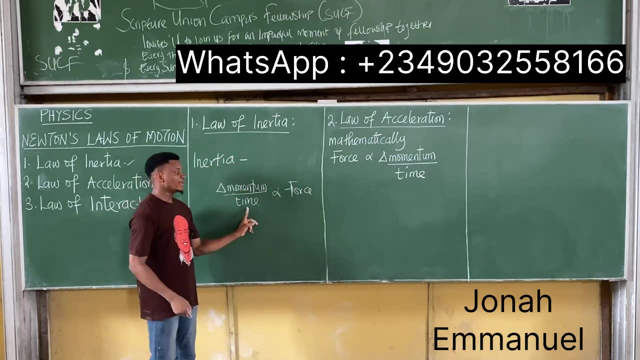 tests being directly proportional to the force. so if I should consider that I should be having change in momentum, or perhaps rate of change of momentum being directly proportional to force, this is what I should have. I should have that rate of change of momentum is directly proportional to force. But how come I now have in 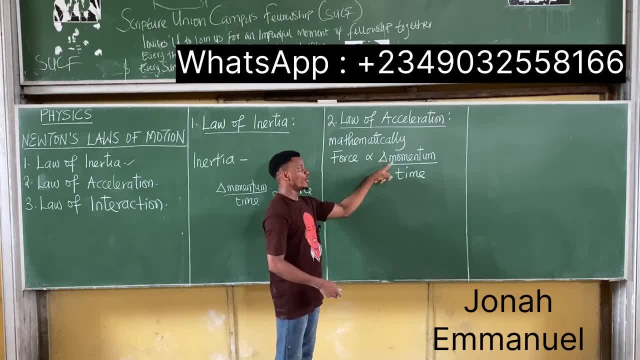 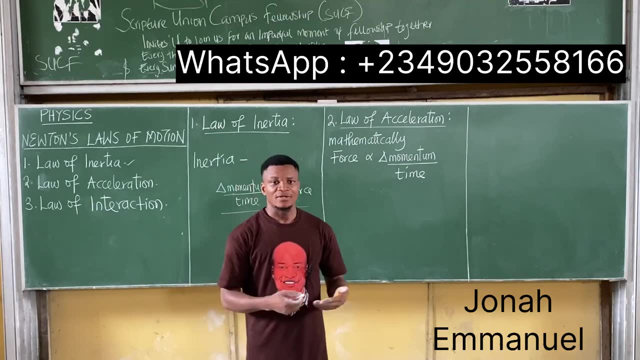 the mathematical expression. how come I now have force before rate of change of momentum? From my definition I'm supposed to have this, But then, in a mathematical form, I am placing the force before the rate of change of momentum. Why is it so? The simple idea is this: There can be no 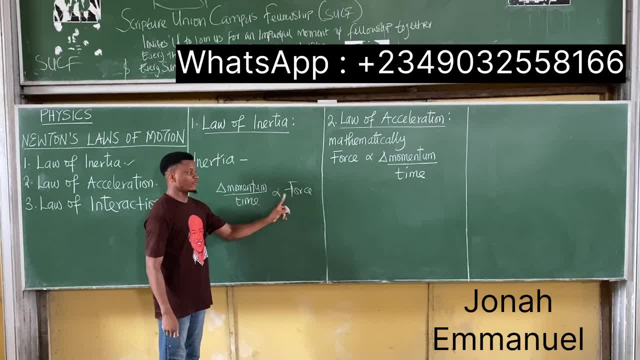 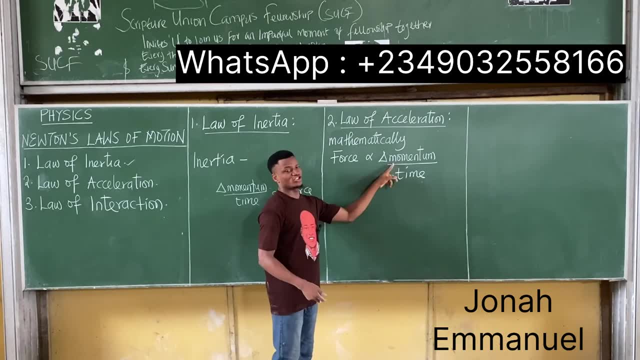 rate of change of momentum is directors, not the force. but how come- and I now have in the mathematical expression- how come I now have force before rate of change of mental? from my definition I am going to have this, but then in a mathematical form I am placing the force before the rate of change of momentum. 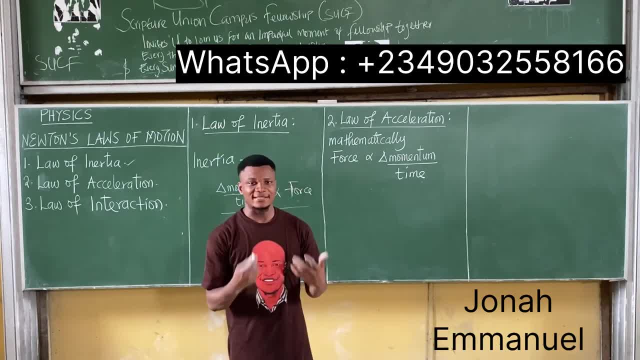 why is it so? the simple idea is this: there can be no rate of change. there can be no change in the 인터� 80 body without an applied force. you can just change to it, but then in a map of a body with an applied force and a force before the rate of change of momentum. why is it so? this simple idea is this: there can be no rate of change in the mentalő. 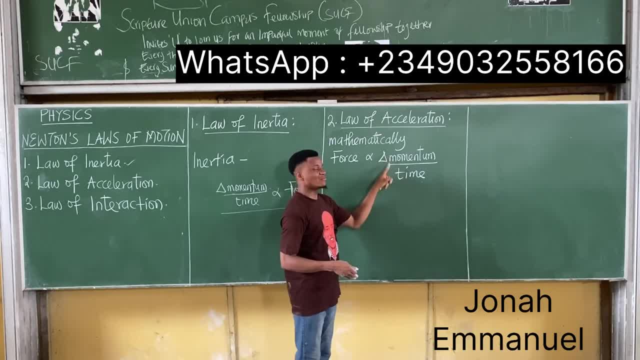 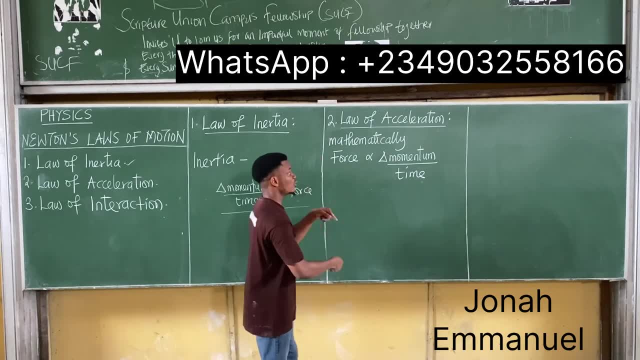 So, before there could be any change in momentum of a body, a force must first be applied. Now this one here gives us, or takes us back to the idea of inertia, or law of inertia, which says that a body will continue in its state of rest or in its uniform motion, except it's been applied or affected by what. 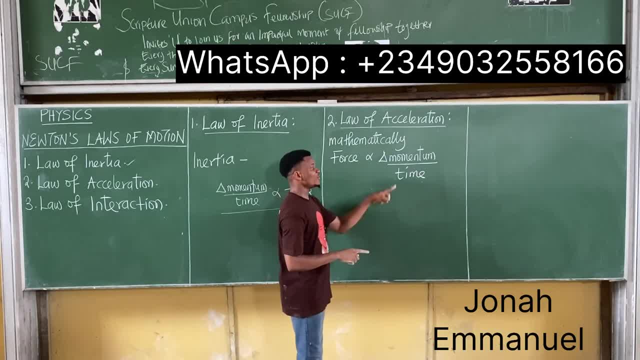 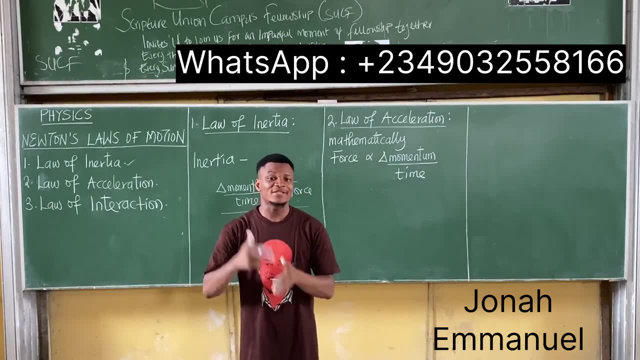 An external force. So in a real sense there can be no rate of change of momentum if a force is not applied. That means in a real sense or in a real world a force must first be applied before there can be a change in momentum. 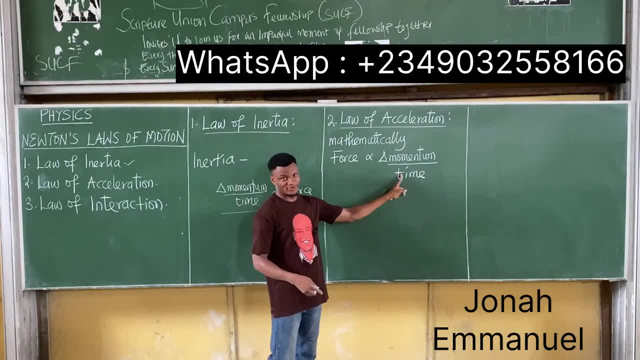 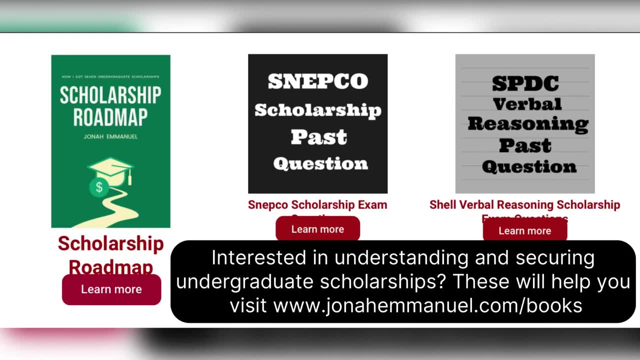 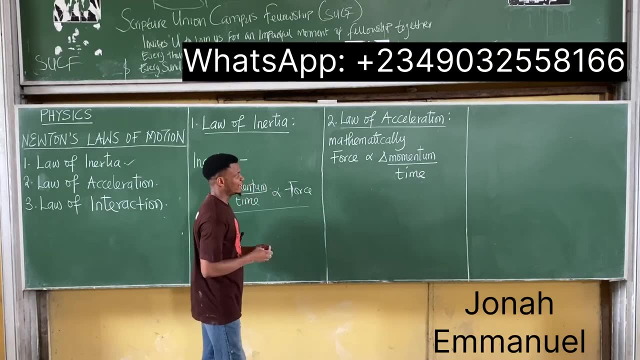 So that's why we place force before momentum. All right, So that's the idea. This is why we swap this. So you have to understand this concept, All right. So Moving on, Moving on. What do we have From here? we have that force F is directly proportional to change in momentum. 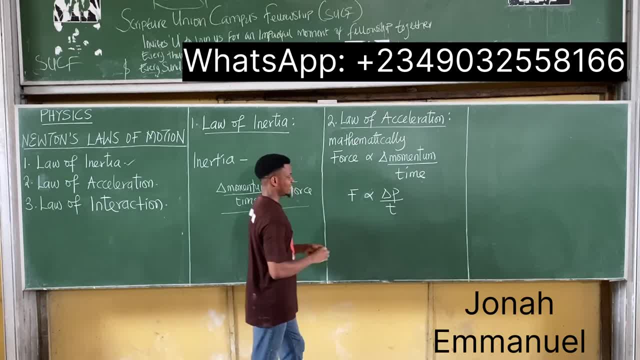 That's this all over time. See, that's this. Now, if this is true, we know that, when it comes to science, to take off the proportionality sign, Right, I'll introduce an equal to and a constant, which, in this case, will have that F. 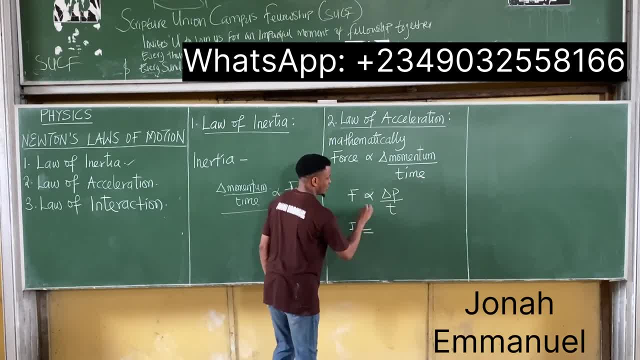 I'll take this off. I'll put an equal. I'll put an equal to and a constant. The constant here will be K. It becomes equal to K. This 2 replaces this one here. Bring back this down. It becomes change in momentum all over time, which is rate of change of momentum. 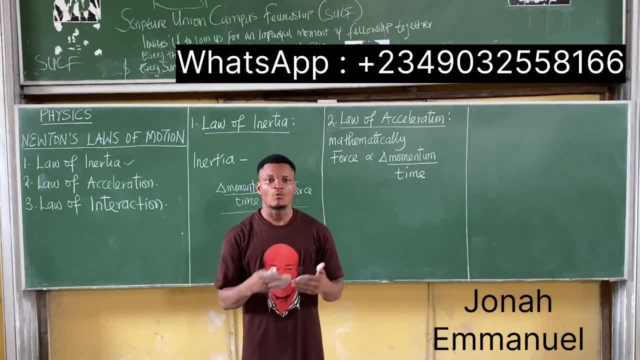 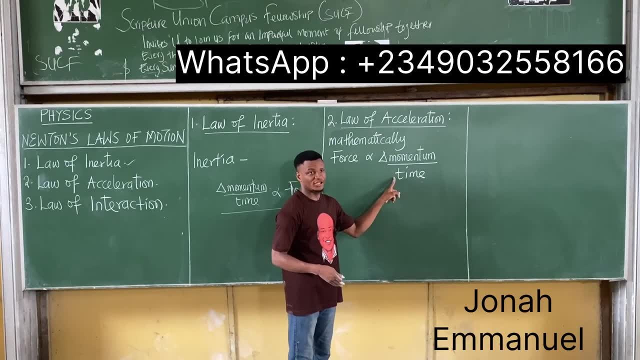 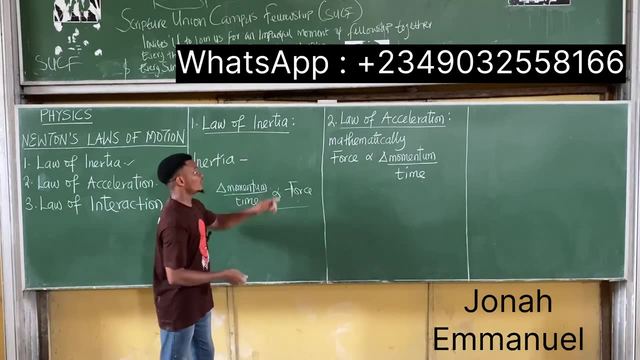 change in the momentum of a body without an applied force. So before there could be any change in momentum of a body, a force must first be applied. Now this one here gives us, or takes us back to the idea of inertia, or law of inertia, which says that a body will continue in its state. 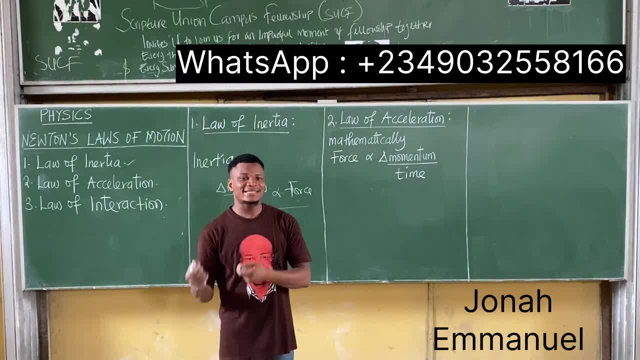 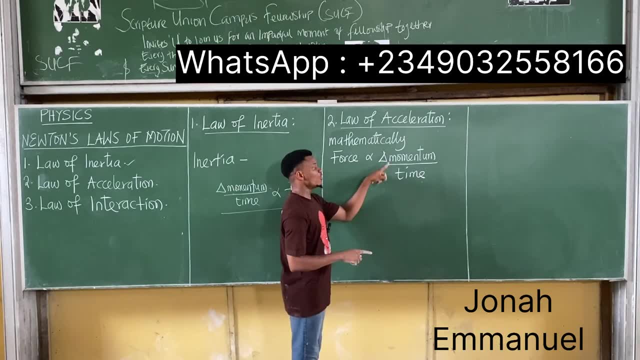 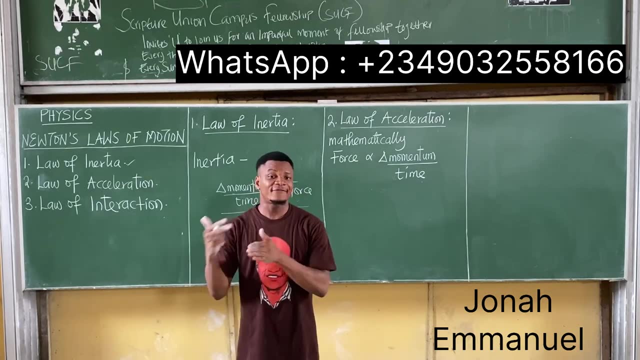 of rest or in its uniform motion, except it's being applied or affected by what An extrapolation force. So in a real sense there can be no rate of change of momentum if a force is not applied. That means in a real sense or in a real world. a force must first be applied before there can be. 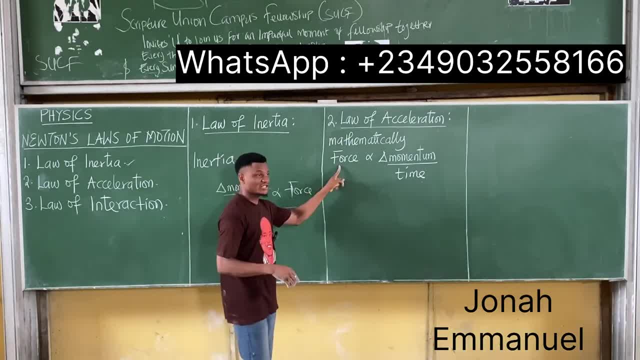 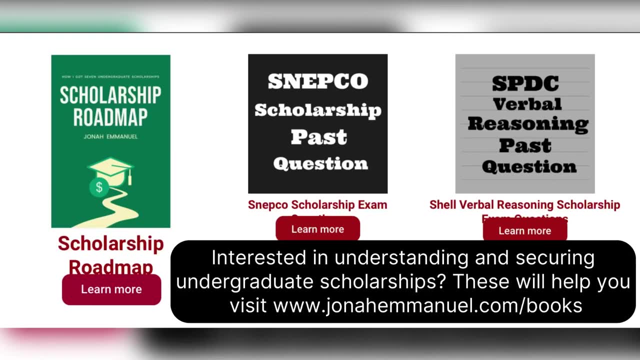 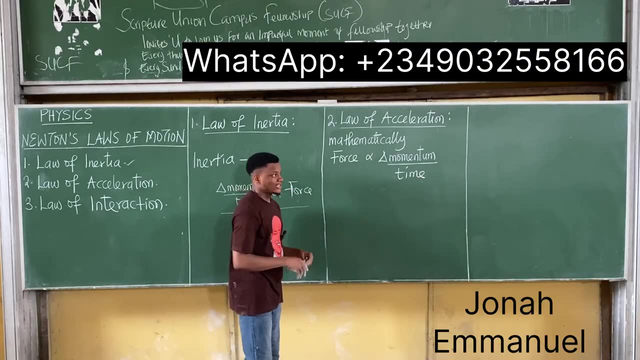 a change in momentum. So that's why we place force before momentum. all right, So that's the idea. That's why we swap this. So you have to understand this concept, All right, so moving on, moving on, what do we have From here? we have that force F is directly proportional to change in momentum. 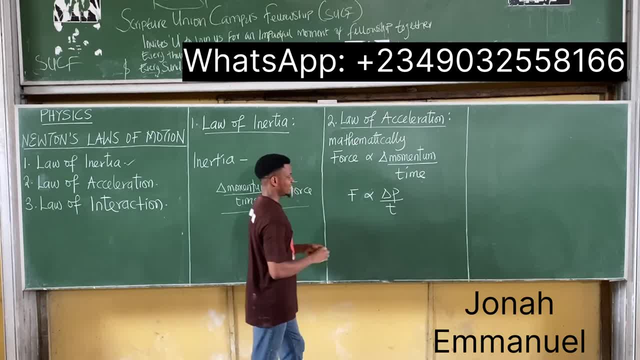 That's this all over time. C. That's this. Now, if this is true, we know that when it comes to science, to take off the momentum, we have to take off the momentum, So we have to take off the proportionality sign. right, I'll introduce an equal to and a constant, which, in this case, 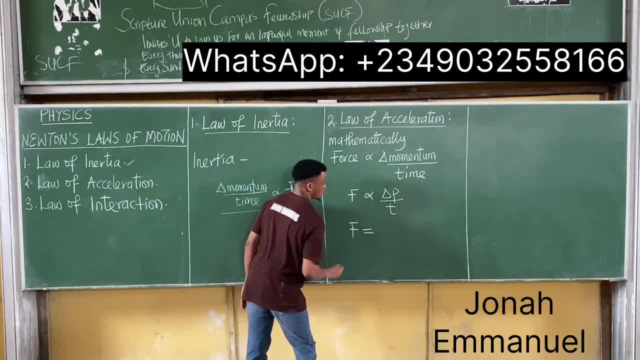 we'll have that F. I'll take this off. I'll put an equal to and a constant. The constant here will be K. It becomes equal to K. This two replaces this one here. bring back this down. It becomes change in momentum all over time, which is rate of change of momentum. 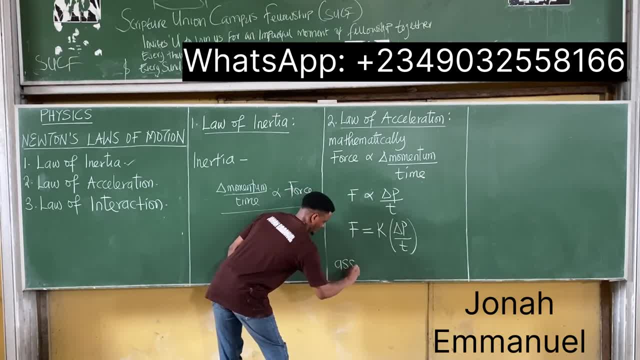 For this one here, we'll assume- let's assume- that the constant K is unity. By unity I mean, let's assume that K is one, That's unity, okay. So when we say unity in science, we mean one. If K is one, what do we? 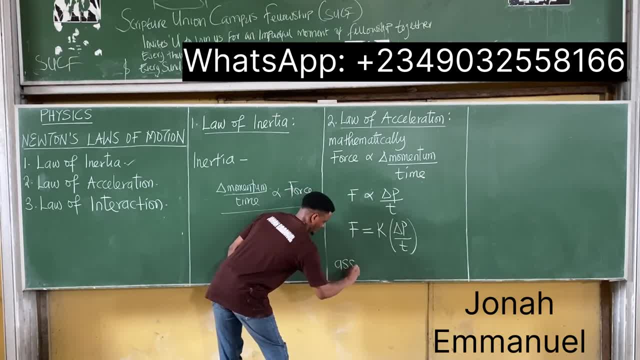 For this one here we'll assume- Let's assume- that the constant K is unity. By unity I mean, Let's assume that K is 1.. That's unity, Okay. So when we say unity in science, we mean 1.. 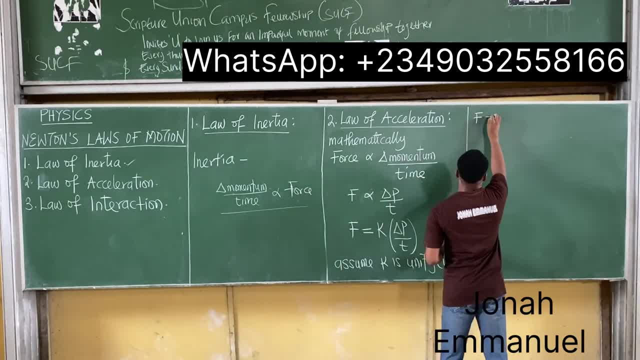 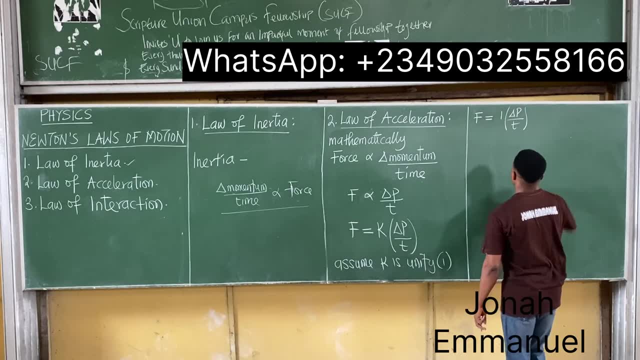 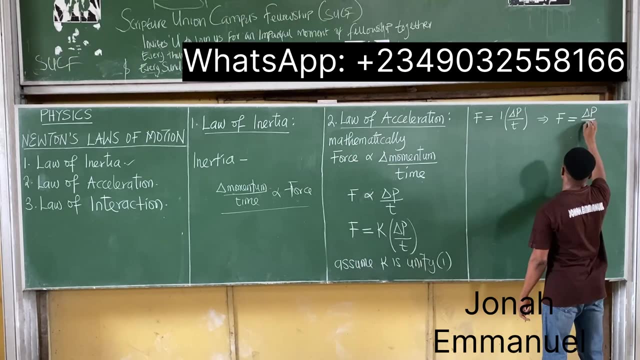 If K is 1, what do we have? We'll have that F is equal to K, which is 1, into changing P all over C. So from here we'll have that F is equal to 1 times. this gives you change in momentum all over time. 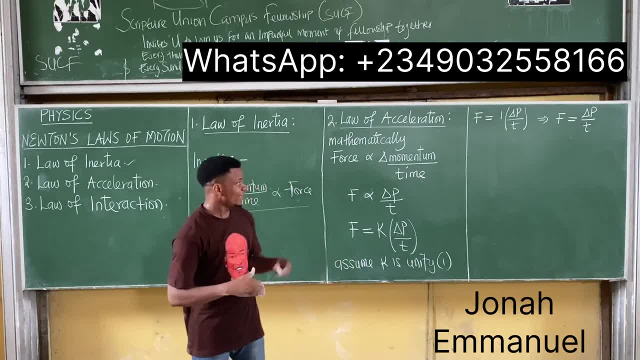 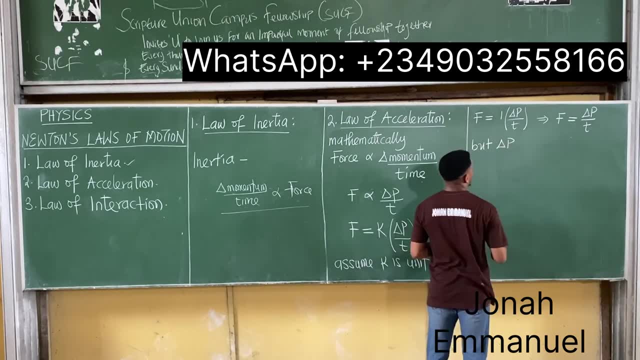 All right. So we are now at this juncture, Let's move on, Let's move on, Let's move on. But So when we say change in momentum, what does it mean? Change in momentum is simply the difference between the final momentum and the initial. 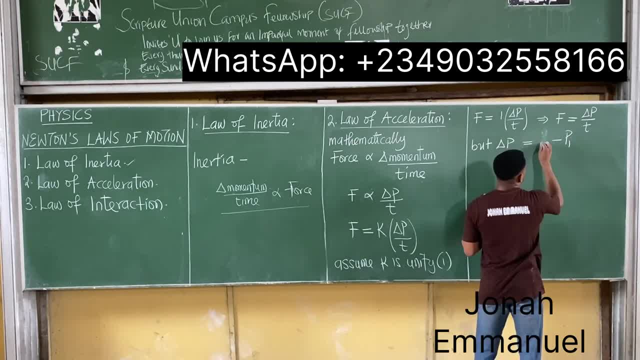 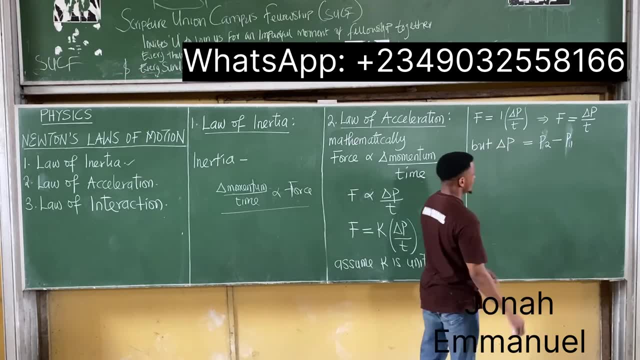 momentum of the body. Okay, Let me use small p. Okay, P2 minus P1.. This is change in momentum, Right, Basically. So I have this. So the difference between the final and initial momentum gives us change in momentum. 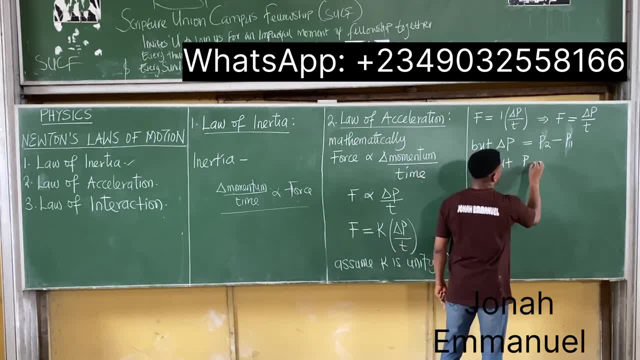 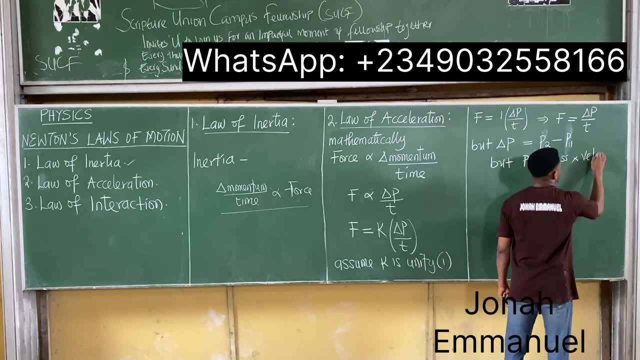 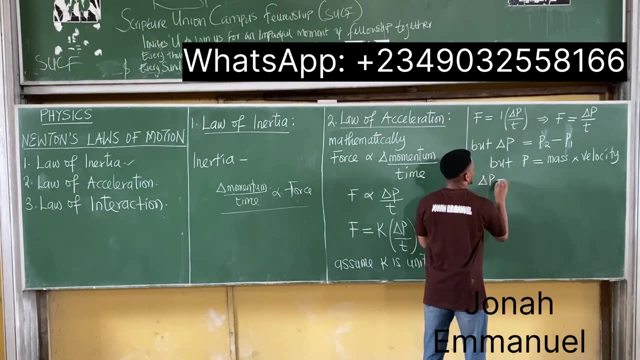 But We said momentum in our previous class is equal to product of mass and velocity. All right, Momentum is equal to product of mass and velocity. So it means that the change in momentum is equal to P2 becomes mass. Since this is the final momentum, it becomes times. 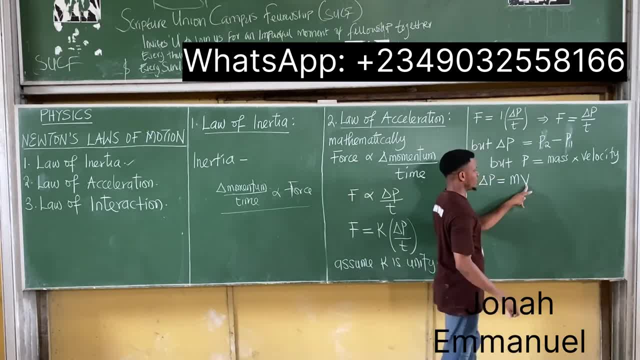 Let's call this V. All right, We'll call this V. V is equal to final velocity Minus P1 is mass times. The velocity for one becomes U, which is initial velocity. So P, we said, is mass times velocity. 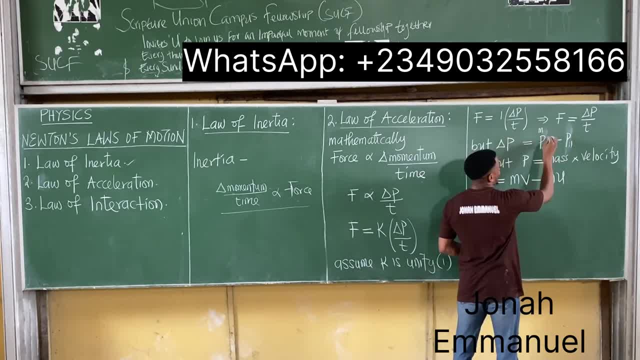 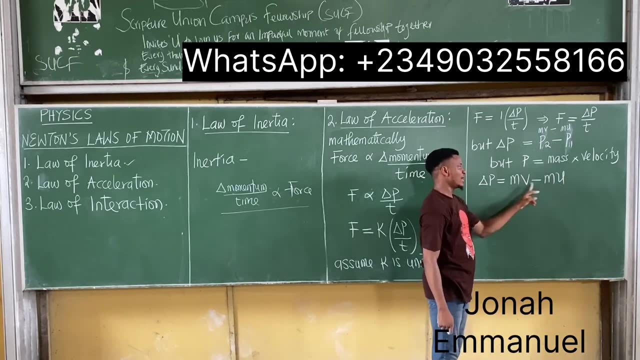 In this case it becomes mass times. final velocity minus This becomes mass times 1. That's initial U, Initial velocity. This is what I have here. Now observe that there's no 1 and 2. Effective- Effective. 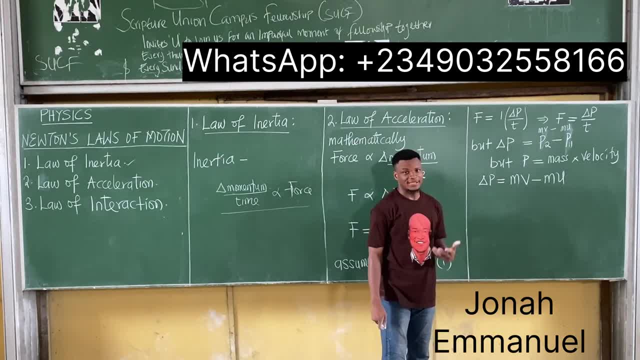 Why? Because the mass of a body is always constant. So the mass of a body is always a constant. That's why we don't have m1 and m2.. It's always constant. If this is true, we'll have that. this is equal to. 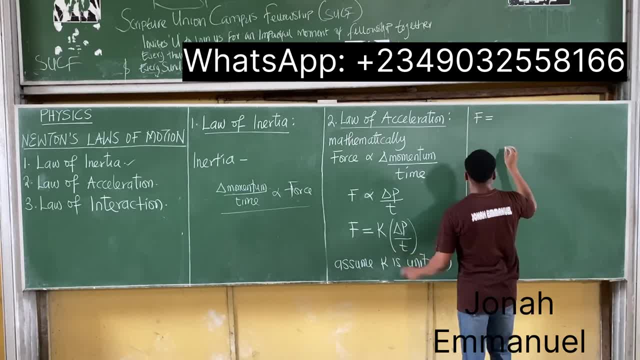 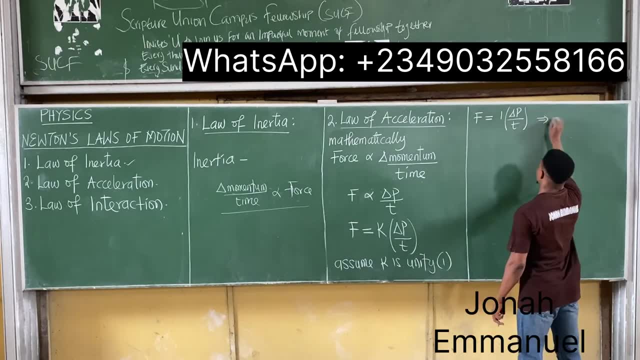 have. We'll have that F is equal to K, which is one into changing P all over C. So from here, we'll have that F is equal to one times. this gives you change in momentum all over time. All right, So we are now at this juncture. 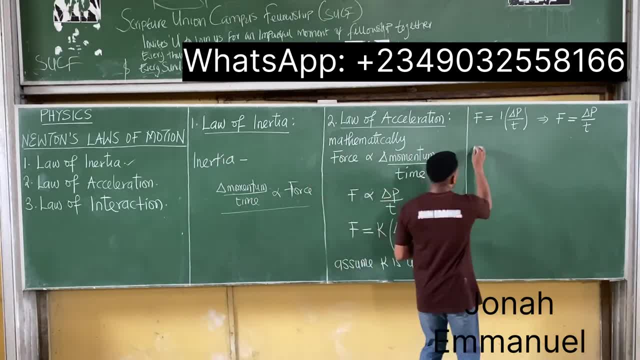 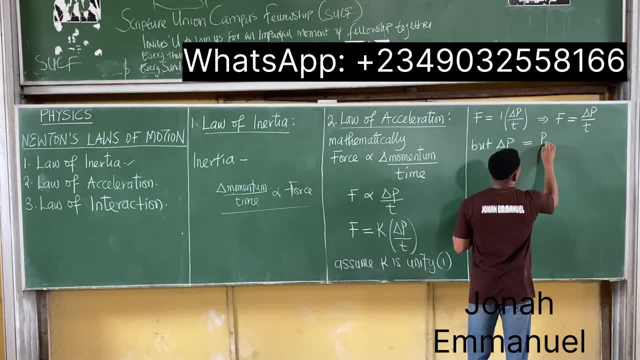 Let's move on, Let's move on, Let's move on. But when we say change in momentum, what does it mean? Change in momentum is simply the difference between the final momentum and the initial momentum of the body. Let me use small p. Okay, P2 minus P1.. This is change in momentum. 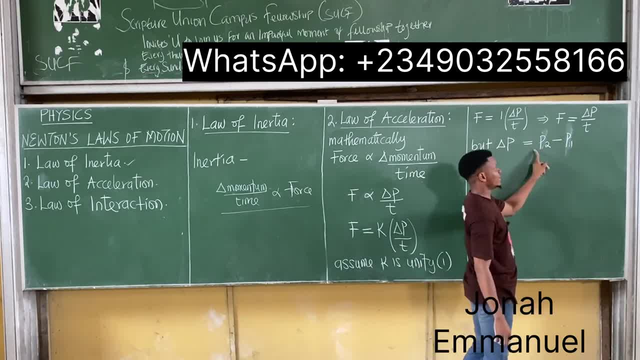 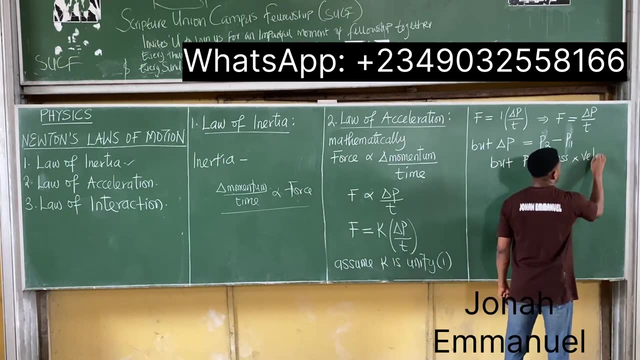 Right Basically. So I have this. So the difference between the final and initial momentum gives us change in momentum. But we said momentum in our previous class is equal to product of mass and velocity. All right, Momentum is equal to product of mass and velocity. 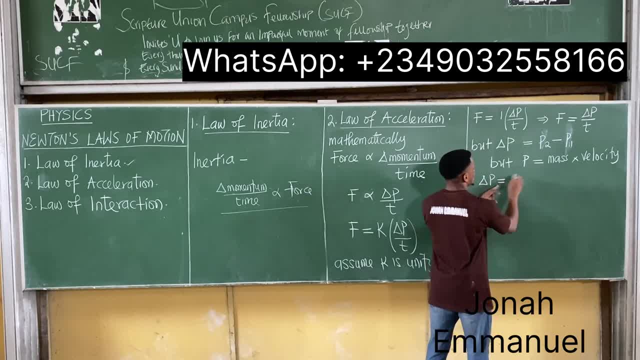 So it means that the change in momentum is equal to P2 becomes mass. Since this is the final momentum, it becomes times. Let's call this V. All right, I'll call this V. V is equal to final velocity minus P1 is mass times the velocity for one becomes U, which is initial velocity, So P. 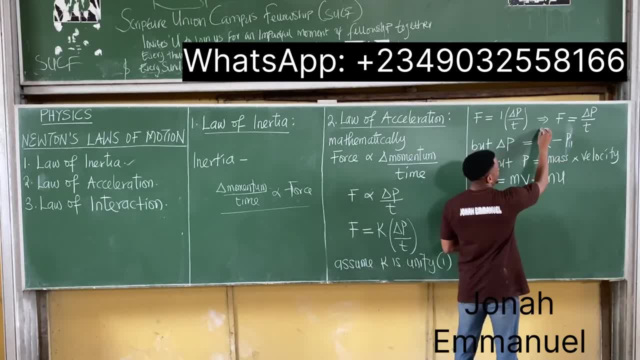 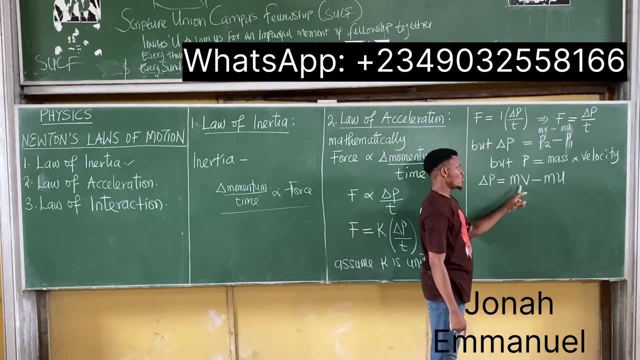 we said is mass times velocity. In this case it becomes mass times final velocity minus. this becomes mass times one. That's initial U, Initial velocity. This is what I have here Now. observe that there's no one and two affecting the masses. Why? Because the mass of a body is always the word constant. So the mass of a body 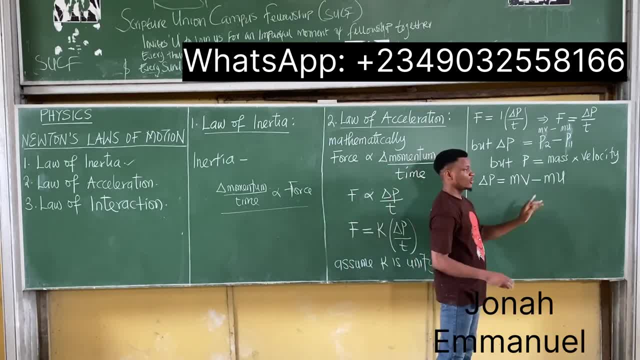 is always a constant. That's why we don't have M1 and M2.. It's always constant. If this is true, we have. this is equal to: I have mass, I have mass. Take off the mass, So bring mass outside. 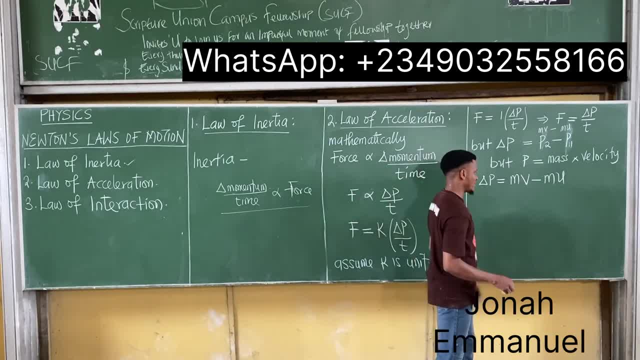 I have mass, I have mass, Take off the mass. So this mass outside, That's factorizing. If I take off mass here I'm left with just V. It becomes V minus Take off mass, here I'm left with just U. 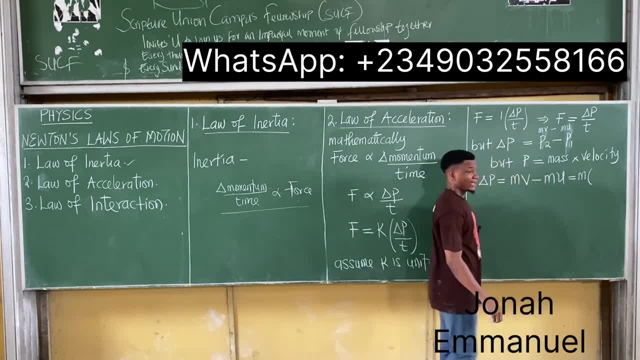 So this is equal to P1 minus. This is equal to P2 minus. This is equal to P3 minus. This is equal to P4 minus. They give you a mass, So this is equal to P. That's vectorizing. 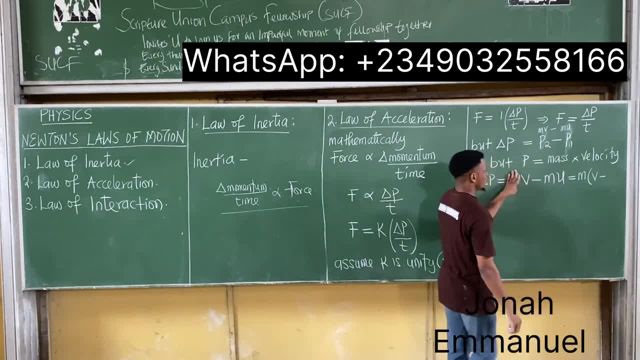 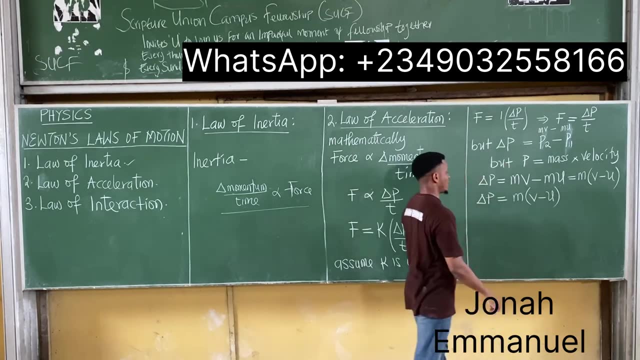 That's vectorizing V minus. take off mass here and let's adjust U So it becomes U. So this means that the change in momentum is equal to mass into V minus U. So I have this Alright. So if this: 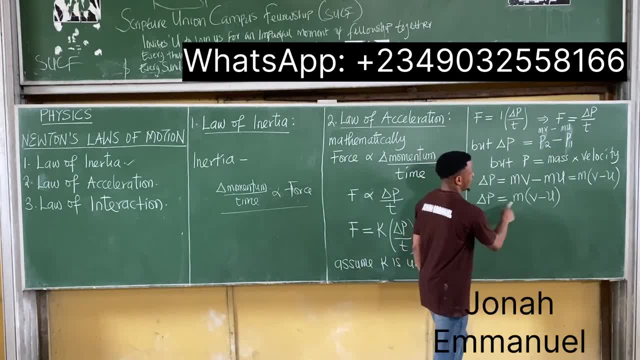 is true. let's fix this idea back into this concept. So we said: force is equal to change in momentum all over time and that's equal to. we just got this value as M into V minus U all over C. So this value is this. I'm doing some mathematical manipulation. We can write: 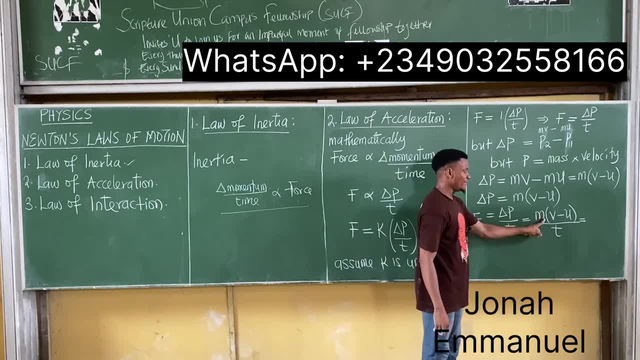 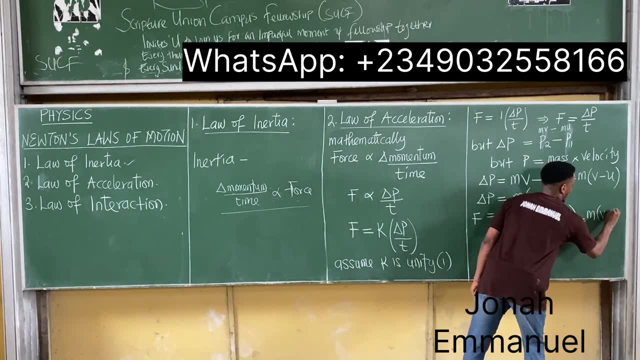 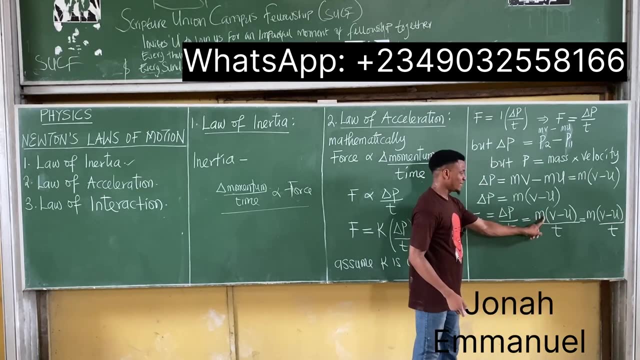 this as being equal to my idea is this: I'll take M out of this so it becomes M into. I'll be left with V minus U, All over T. So please notice what I did From here. I just shifted. the mass outside becomes. 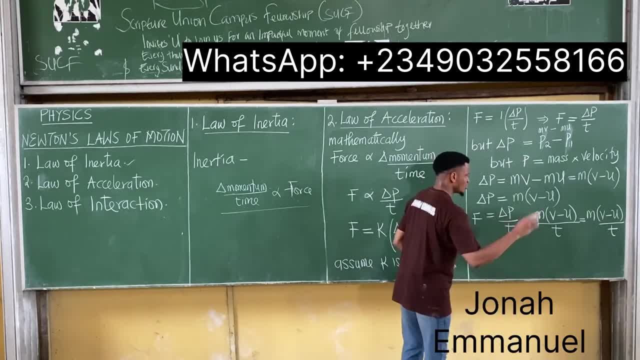 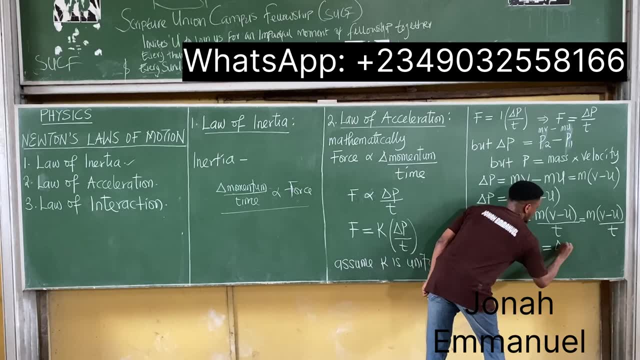 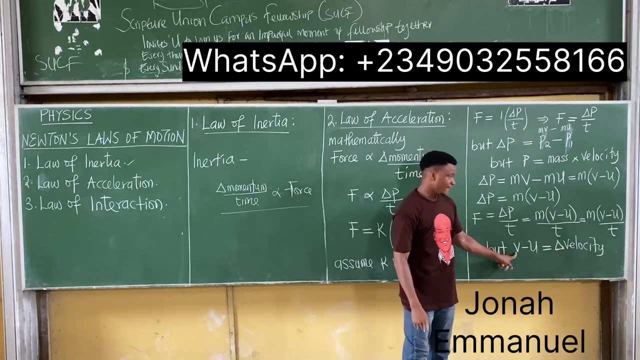 V minus U over T. Now, but something. but we know that V minus U is equal to change in velocity, Of course, Because V means final velocity and U means initial velocity. So you can say that V minus U is equal to change in velocity. So if this is true, what then do we have? 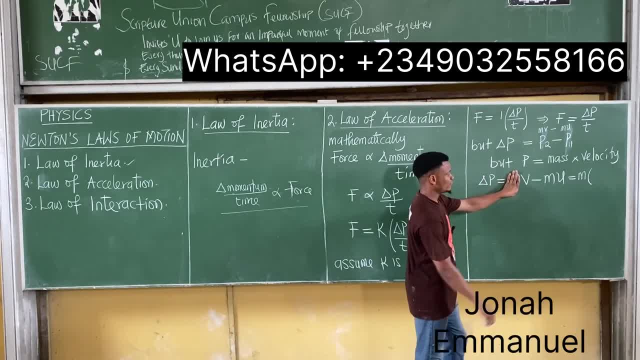 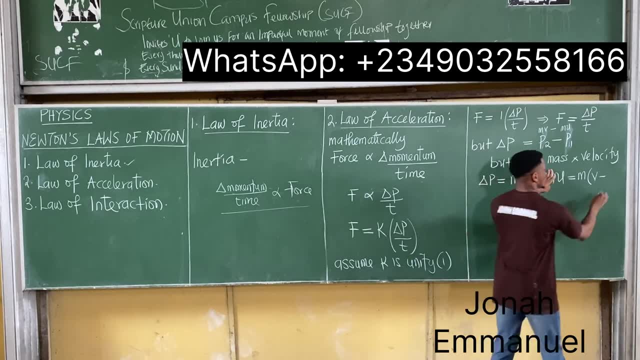 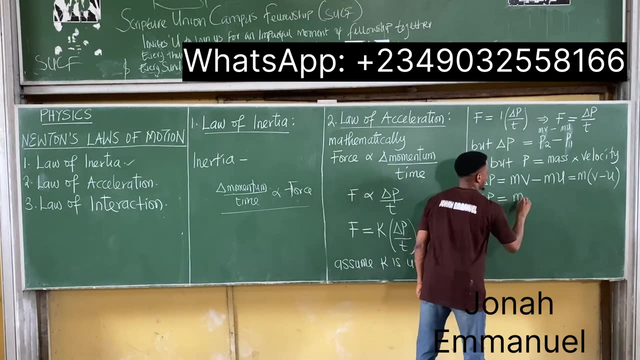 That's factorizing. If I take off mass- here, I'm left with just V, It becomes V minus. Take off mass- here, I'm left with just U, It becomes U. So this means that the change in momentum is equal to mass into V minus U. So I have this. 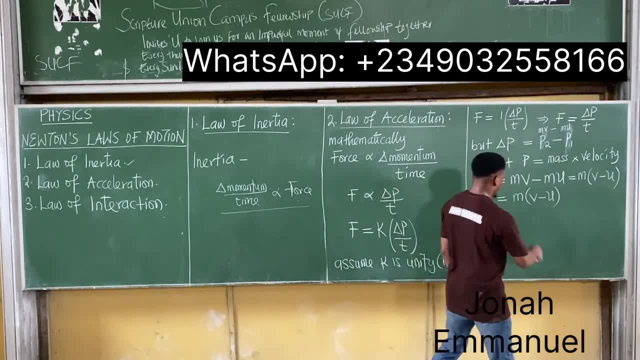 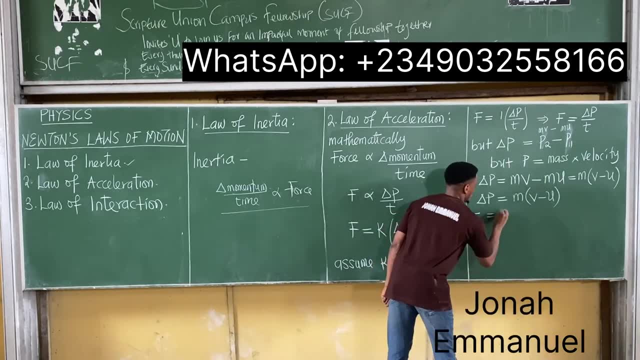 All right. So if this is true, let's fix this idea back into this concept. So we said: force is equal to change in momentum all over time And that's equal to. we just got this value as M into V minus U all over C. So this value is this. I'm doing some mathematical manipulation. We can write this as: 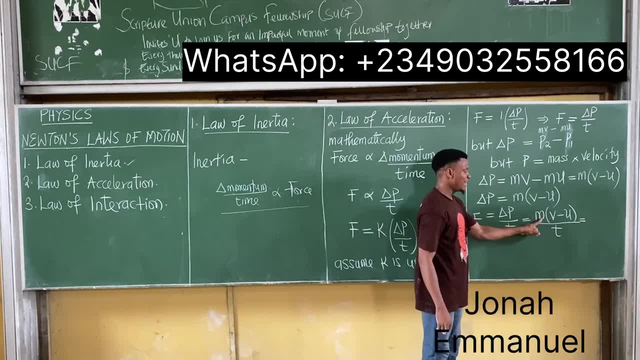 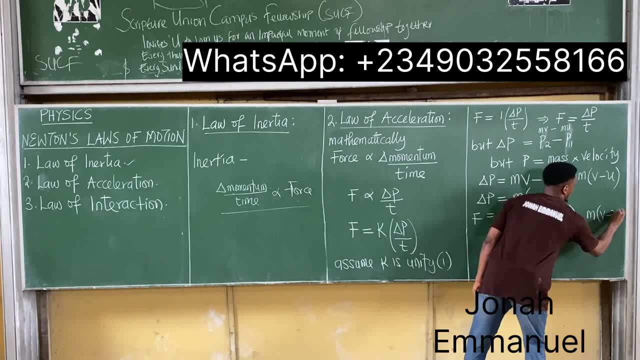 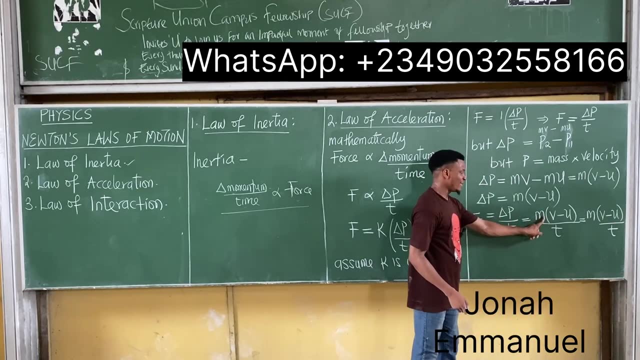 being equal to My idea is this: I'll take M out of this So it becomes M into. I'll be left with V minus U, All over C. So please notice what I did from here. I just shifted. the mass outside becomes. 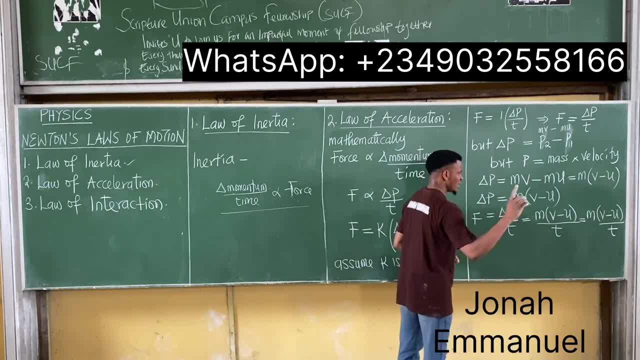 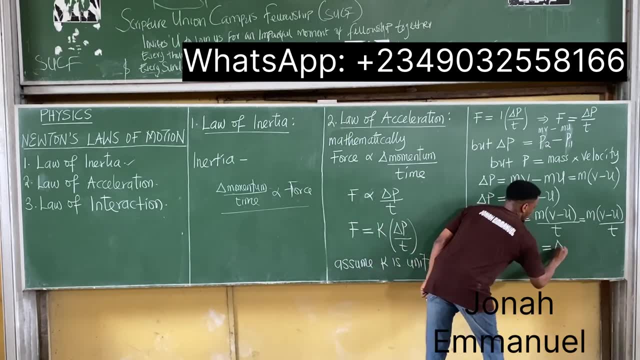 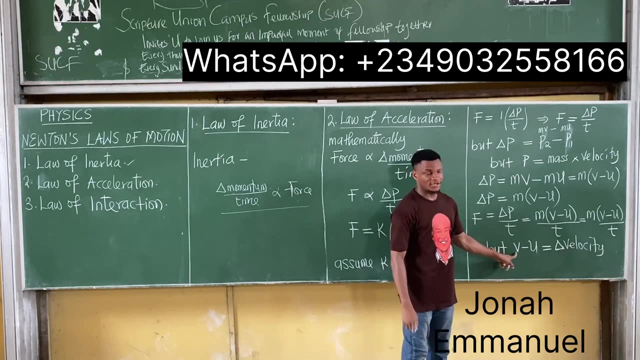 V minus U over T Now, but something. but we know that V minus U is equal to change in velocity, Of course, because V means final velocity and U means initial velocity. So you can say that V minus U is equal to change in velocity. So if this is true, what then do we have? 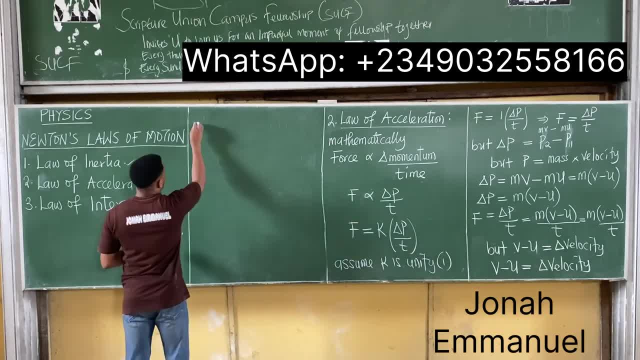 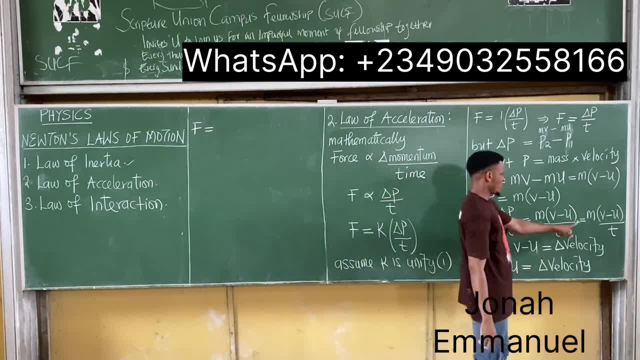 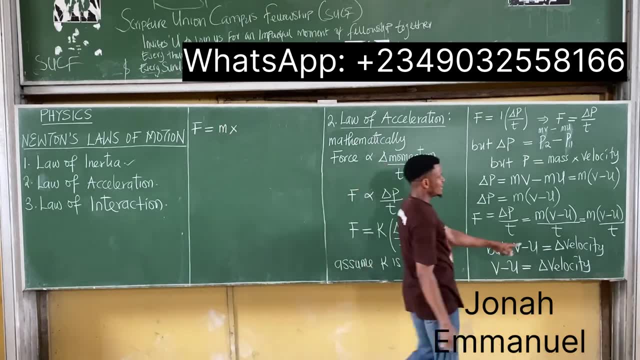 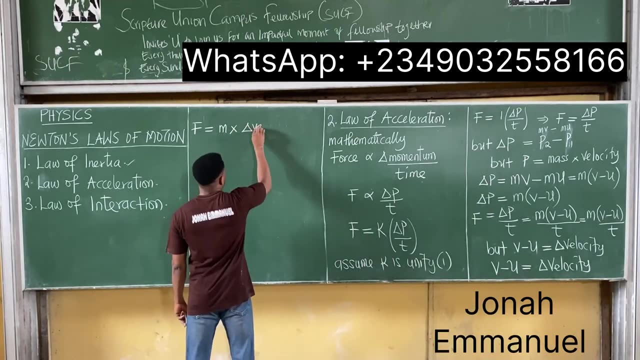 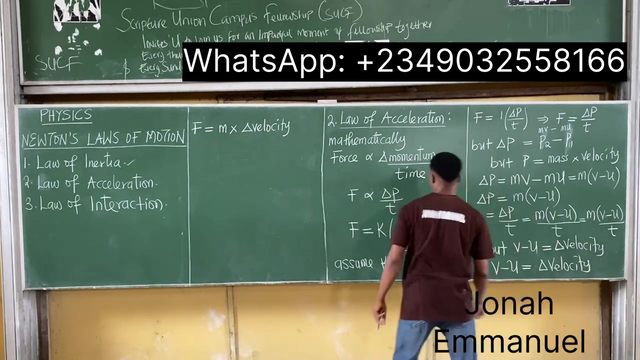 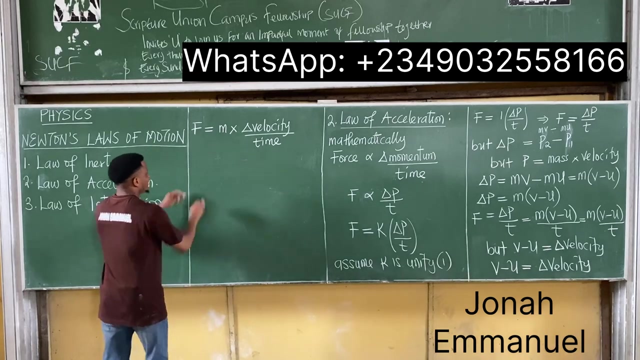 equal to from this point, from this point mass becomes mass times. we just said, V minus U means change in velocity. so first times change in velocity. now, this one here was divided by T, so divided by T, so divided by T, which is time we can use T, or time that's it. but then again, but from the very basics of physics, we 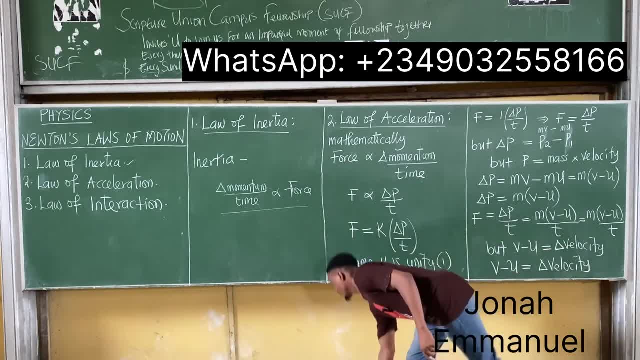 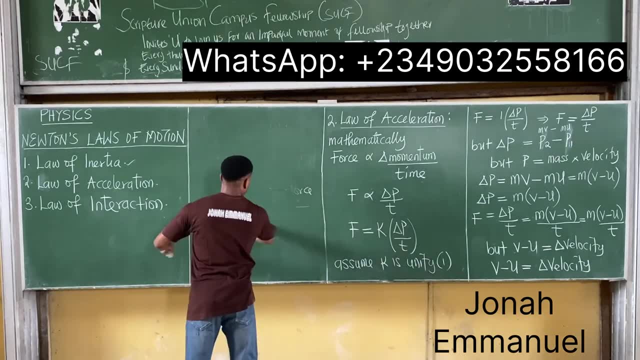 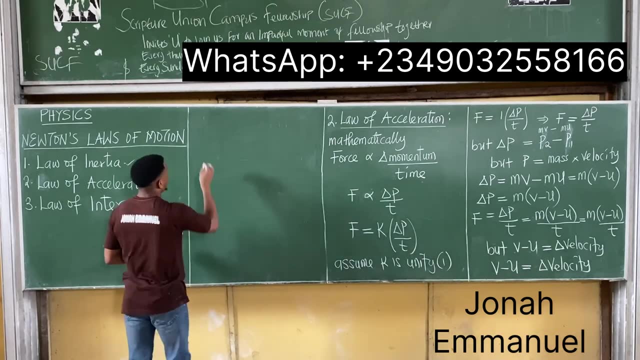 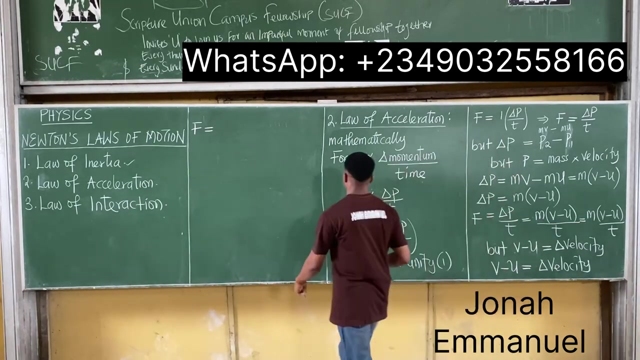 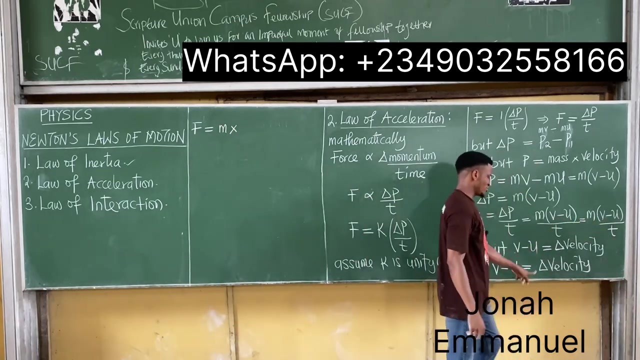 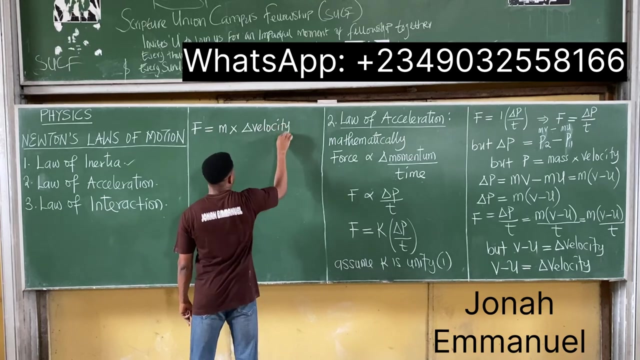 So if this is true, that means we have that uh, force is equal to U plus M into V minus U. It's to from this point. from this point mass becomes mass times. we just said V minus U means change in velocity. so first times change in velocity, now this one. 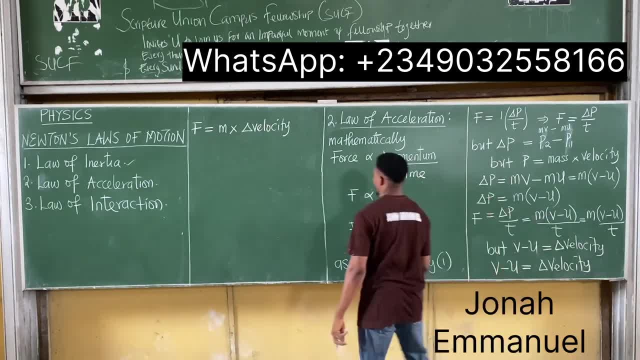 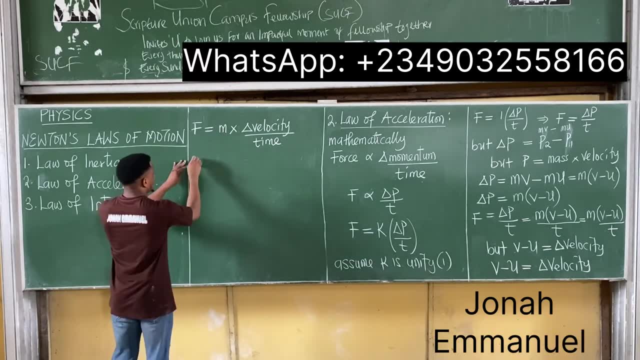 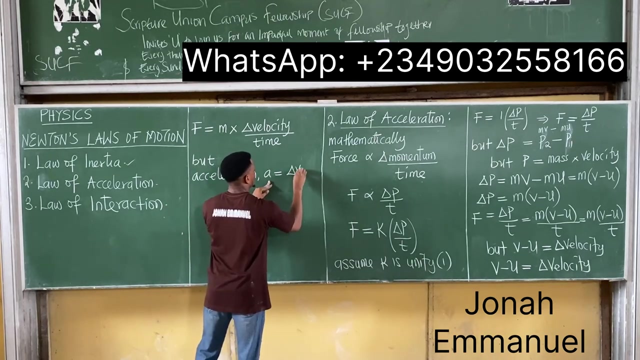 here was divided by T, so divided by T, so divided by T, which is time. we can use T or time, that's it, but then again. but from the very basics of physics we know that acceleration- acceleration that's A- is equal to change in velocity all over. 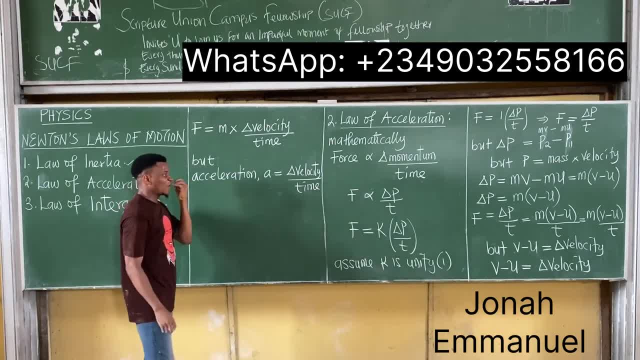 time. all right, because we defined acceleration as the rate of change of velocity. so acceleration is equal to change in velocity over time. if that's true, that means that force is equal to mass. let me write this in: okay: mass times change in velocity over time. we said it's. 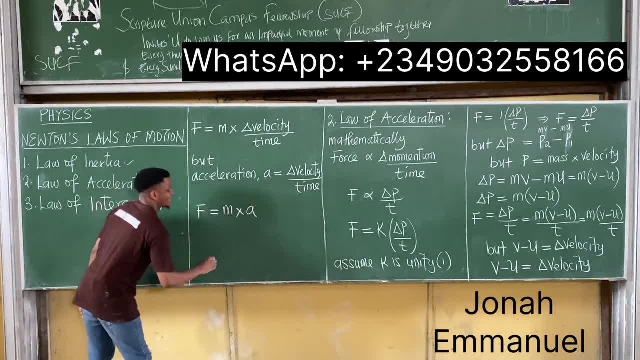 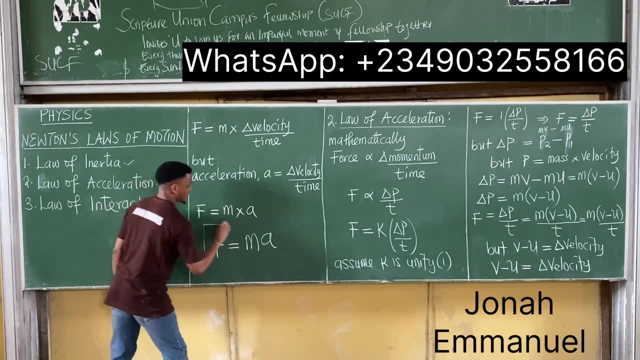 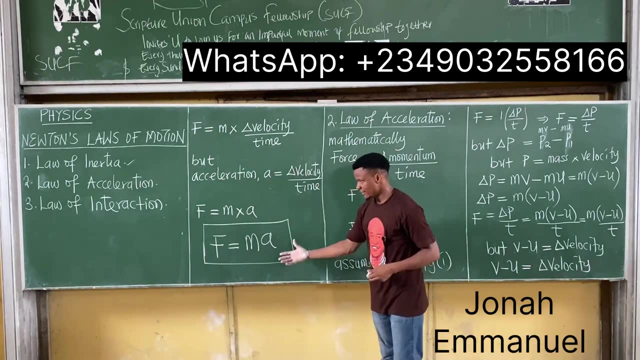 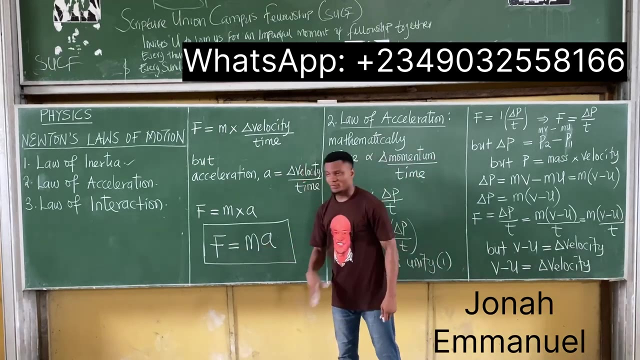 acceleration, that's acceleration. if I combine this, it means that force is equal to mass times: acceleration. this is the mathematical expression of Newton's second law of motion, right? so we have this one here, the very important concept, a very critical concept in physics: that force is equal to the product of mass and acceleration. all right, so let's look at. 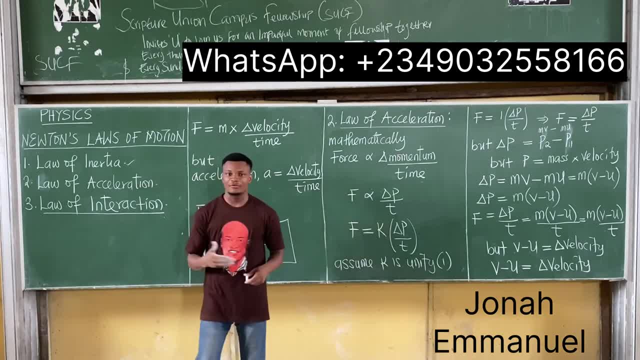 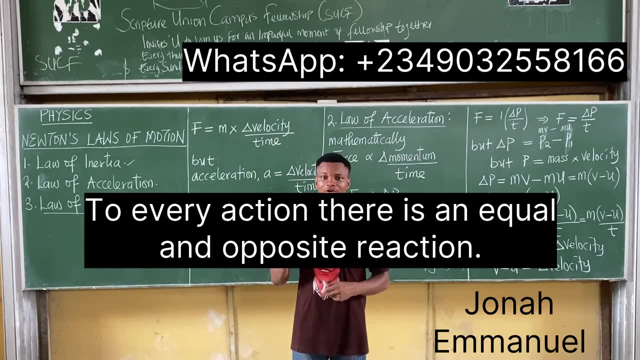 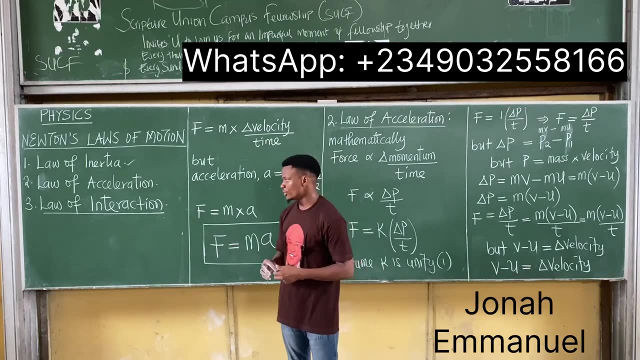 let's look at Newton's third law of motion. it is called the law of interaction, and the law of interaction simply states that to every action there's an equal and opposite reaction. that is the statement of Newton's third law of motion, also called the law of motion. 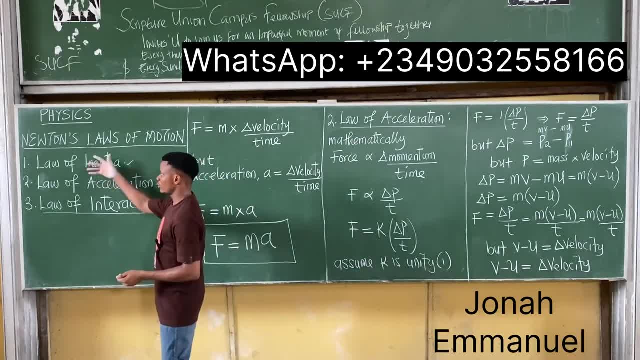 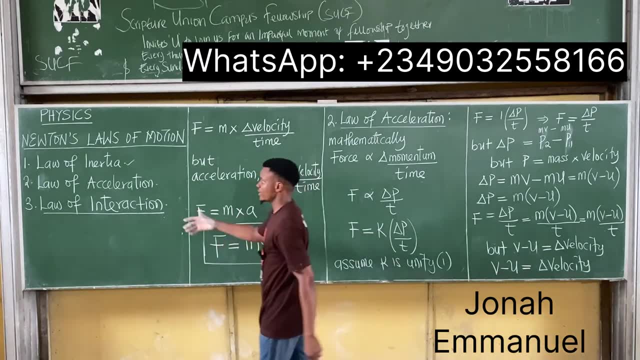 interaction. All right, so we finally discussed all of Newton's laws of motion, law of inertia, law of acceleration and then the law of interaction. So we'll see how we apply the concept, especially the law of acceleration, into the rate of change of momentum or into the law. 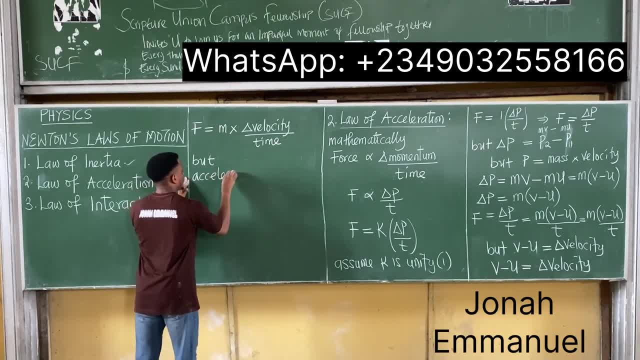 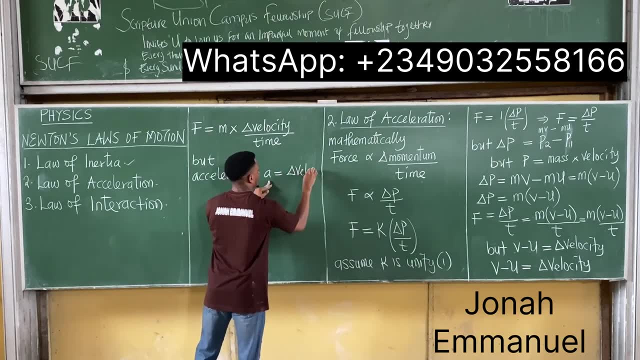 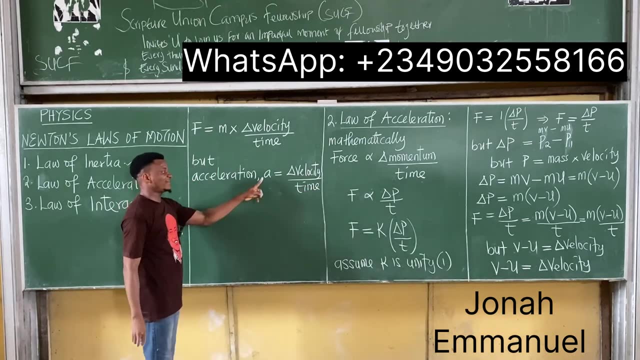 know that acceleration- acceleration, that's A- is equal to change in velocity all over time. all right, because we defined acceleration as the rate of change of velocity. so acceleration is equal to change in velocity over time. if that's true, that means that force is equal to mass. 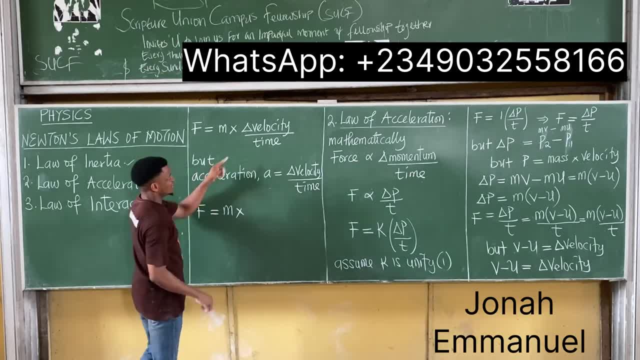 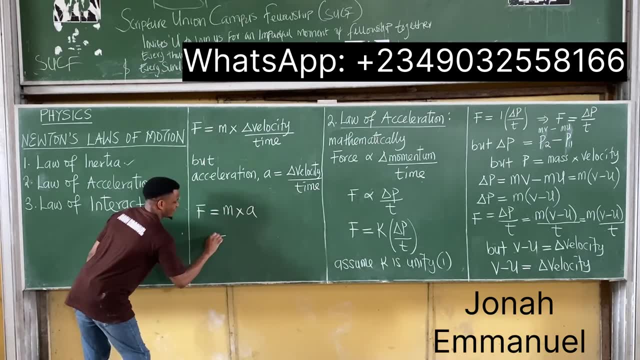 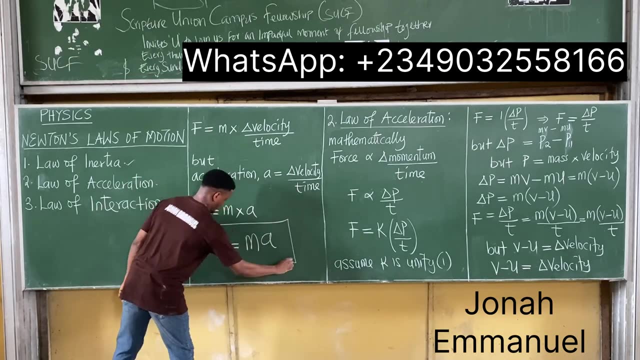 let me write this in: okay, mass times change in velocity over time, we said, is acceleration, that's acceleration. if I combine this, it means that force is equal to mass times acceleration. this is the mathematical expression of Newton's second law of motion. right, so we have this one here. 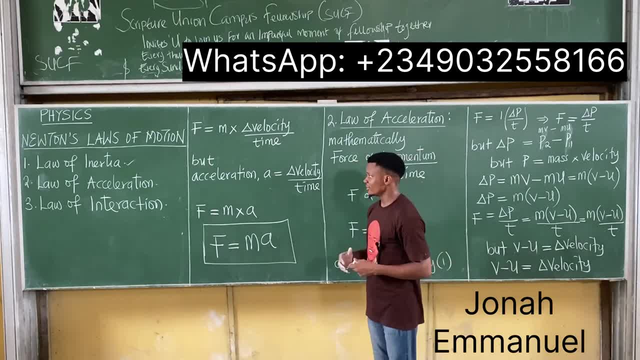 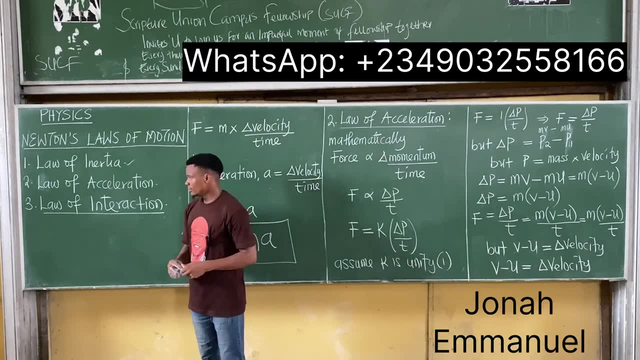 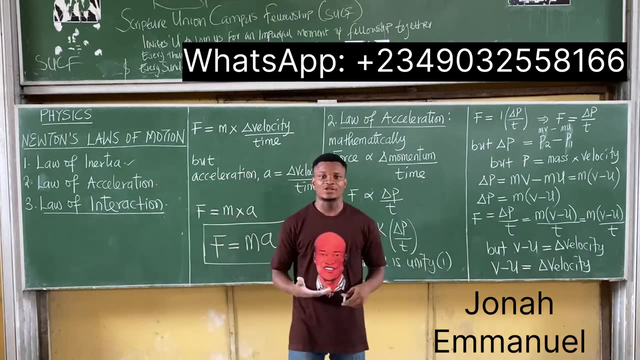 the very important concept, a very critical concept in physics, that force is equal to the product of mass and acceleration. all right, so let's look at Newton's third law of motion. it is called the law of interaction, and the law of interaction simply states that to every action there's an equal and opposite. 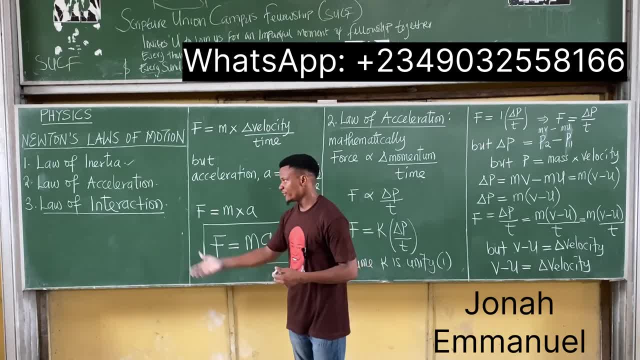 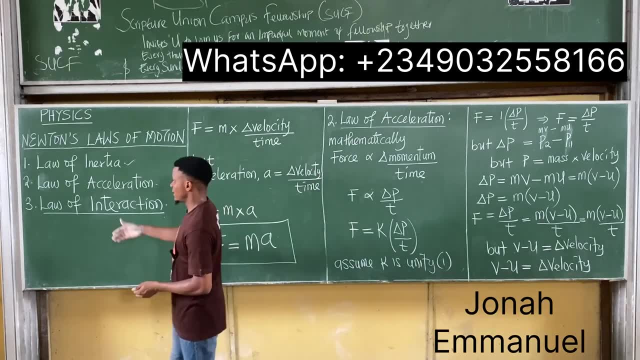 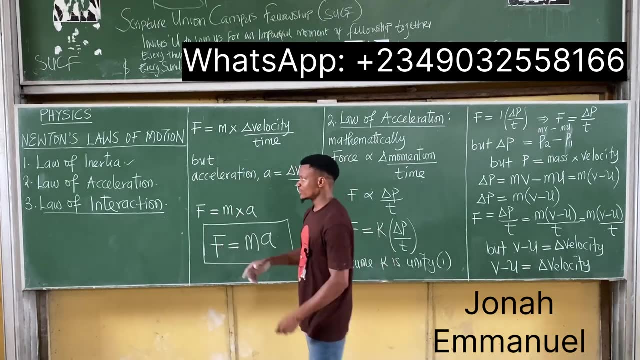 reaction. that is the statement of Newton's third law of motion, also called the law of interaction. all right, so we finally discussed all of Newton's laws of motion: law of inertia, law of acceleration and then the law of interaction. so we'll see how we apply the concept, especially the law of acceleration, into the rate of change of 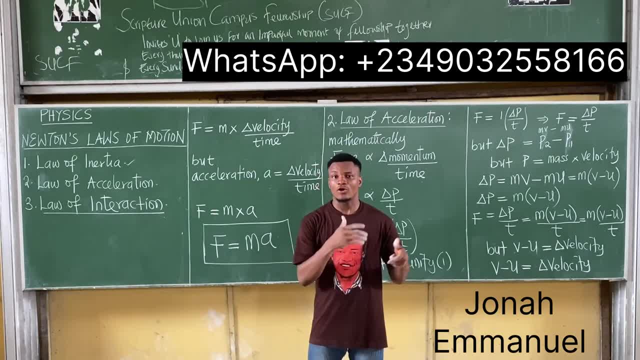 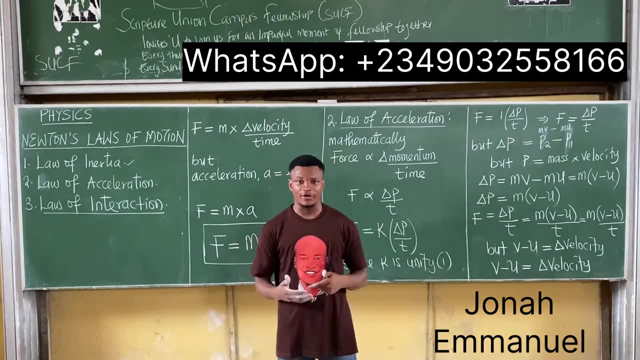 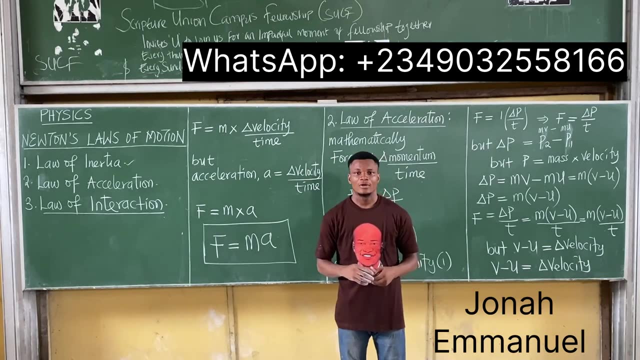 momentum or into the law of conservation of momentum. we'll also look at how to apply the law of interaction into things like the recoil of a gun and etc. all right, and we'll look at this in our next class. okay, all right, so I've made over 50. 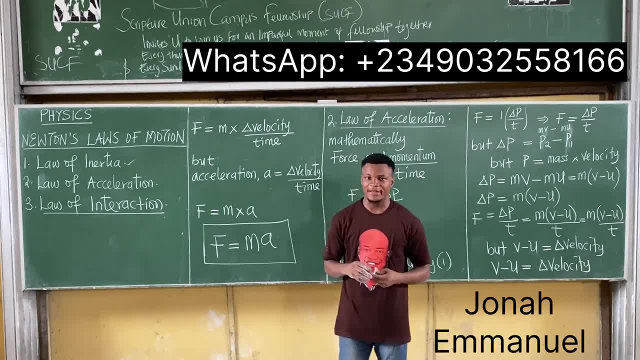 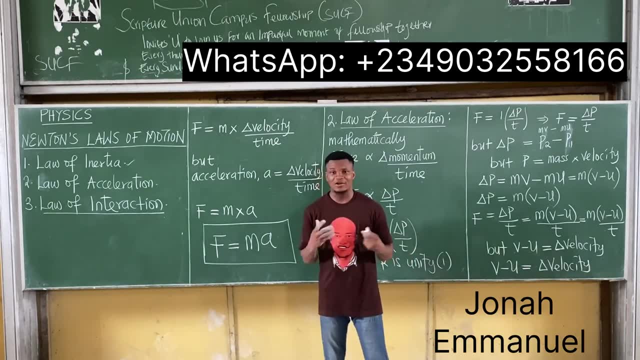 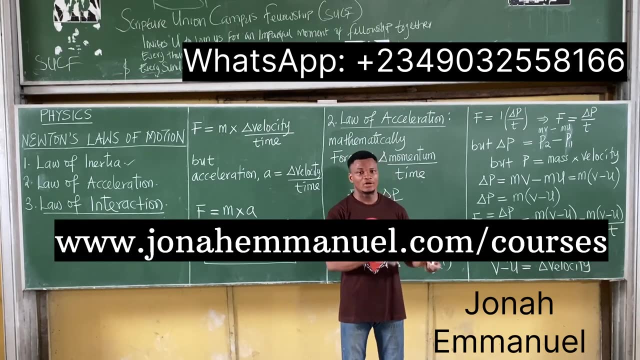 videos on physics, chemistry, mathematics and the other sciences to help you prepare for your yx or jam examination. all right, to get my complete videos on physics, chemistry, mathematics and the likes, please visit my website wwwjohnahemmanuelcom. forward slash courses. then look at the jam.